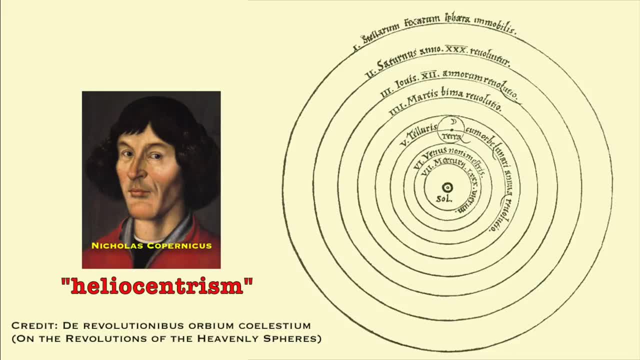 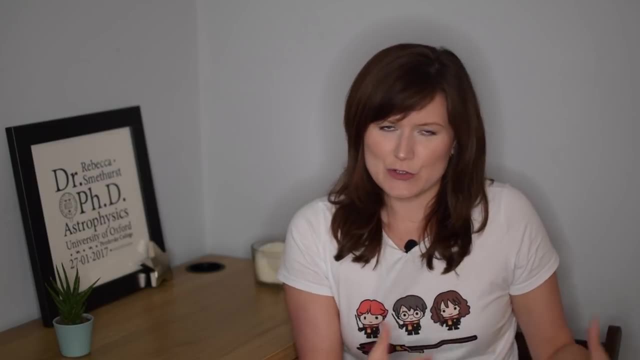 supporters of Copernicus's heliocentrism model. This is when Copernicus placed the sun, and not the earth, as the centre of what was then the entire universe. And in 1584 Bruno made the leap to say: well, if the sun is the centre of our solar system, then perhaps all the other stars in the sky? 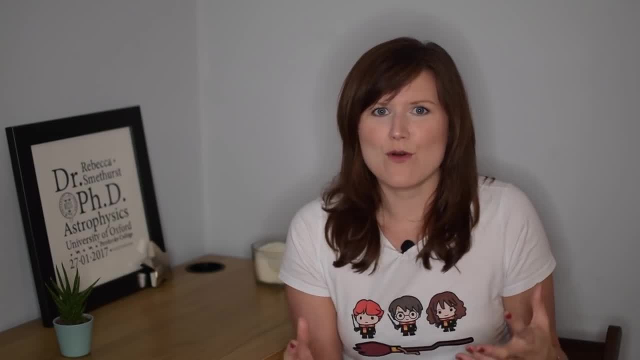 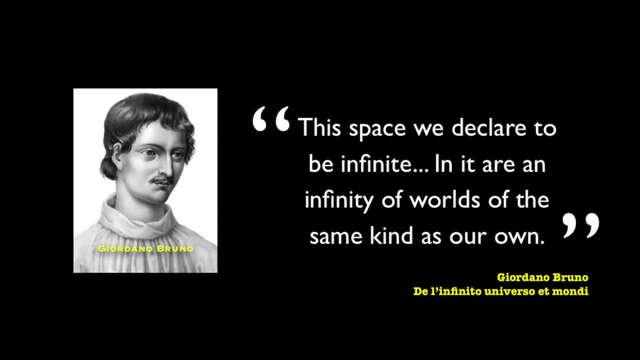 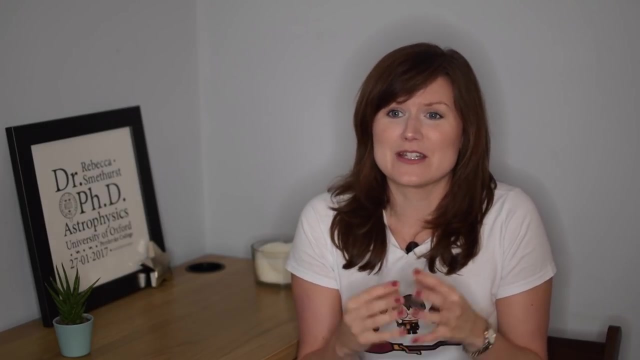 are just like the sun and so therefore also have planets around them as well. In his musings he also insisted that the universe was infinite and had no centre either. So this guy was way ahead of his time, So far ahead that the Catholic church at the time decreed everything. 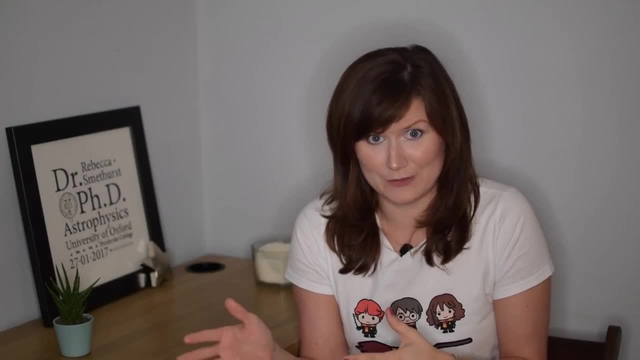 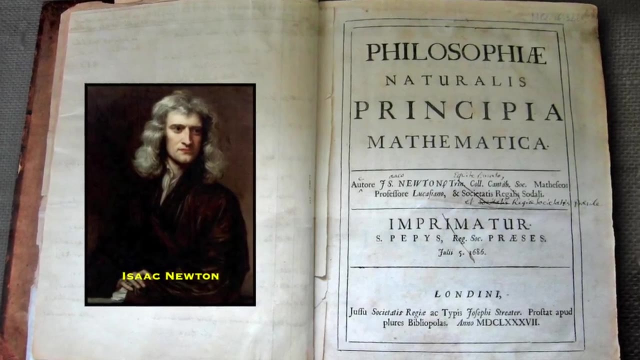 he said as heresy and burned him at the stake for his beliefs. Fast forward now to the 18th century and the publication of Isaac Newton's Principia in 1713. One of the most famous books of the 18th century. 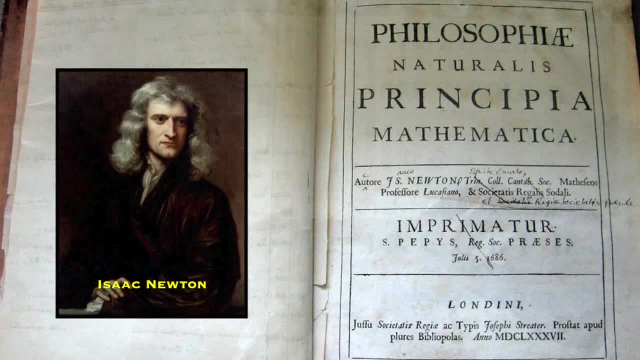 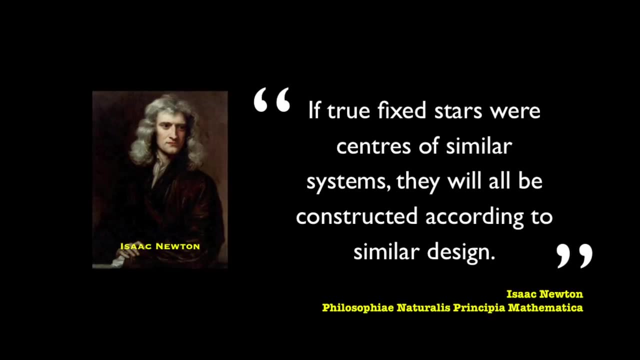 It's one of the most famous books of the 18th century. It's one of the most famous scientific works ever, In the conclusion of which Newton, comparing stars in the sky to the sun, he said: if true, fixed stars were centres of similar systems. 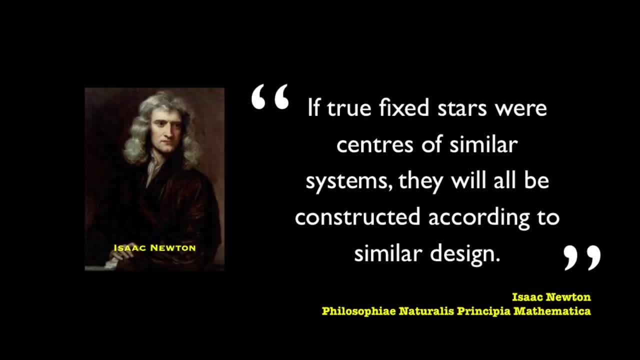 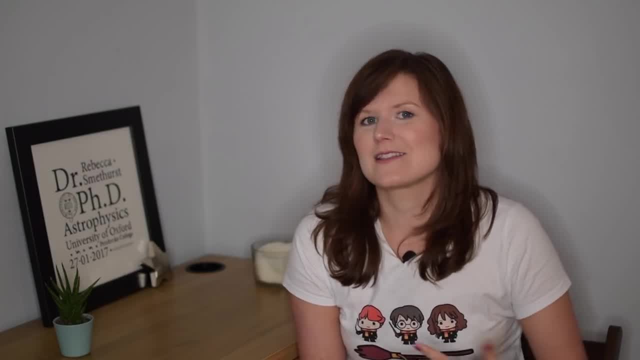 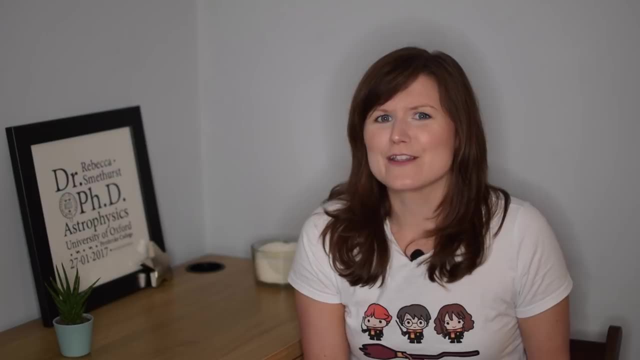 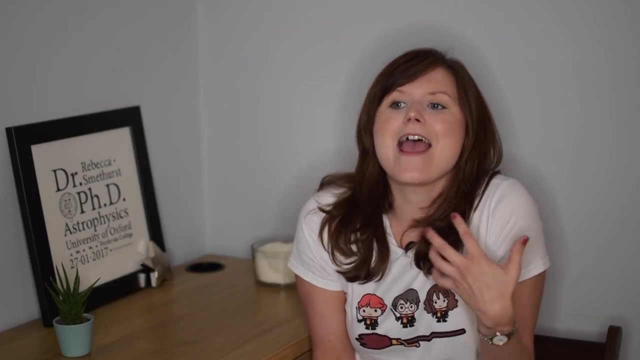 they will all be constructed according to similar design, aka the stars in the sky should also have planets in them. And for Newton to echo that same belief, it really fixed in people's minds that the sun wasn't alone in the universe. Of course, you have to then prove that that is the case, and so everybody wanted to be the first person. 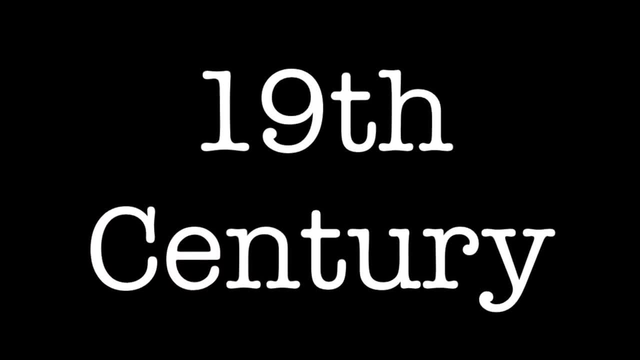 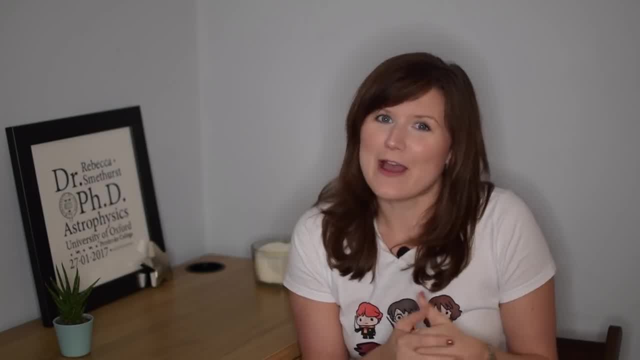 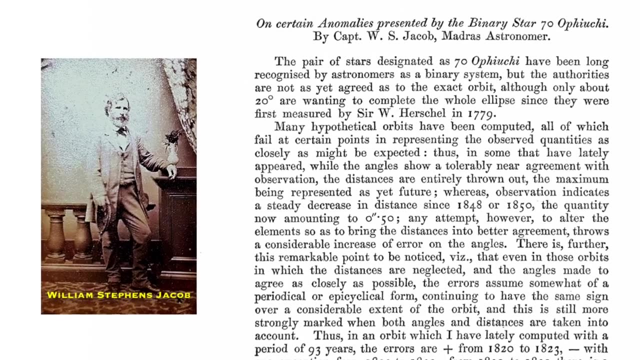 to detect an extra solar planet And as telescopes got better towards the end of the 19th century, one of the first claims- albeit a false claim- of exoplanet detection came through When William Stevens Jacob, as early as 1855, announced that he'd discovered a planet around. 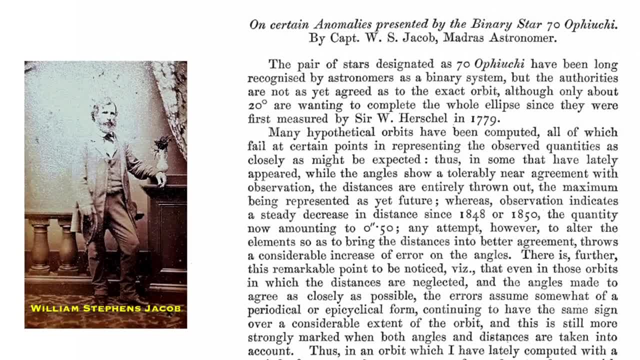 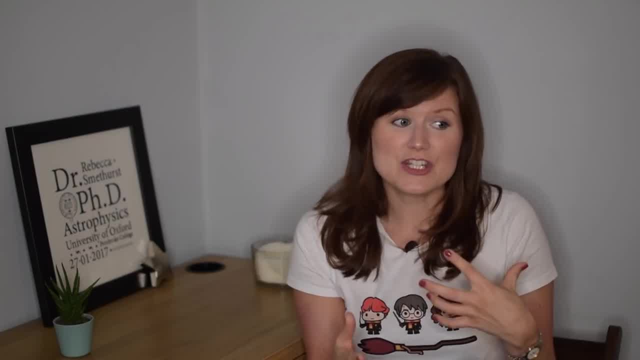 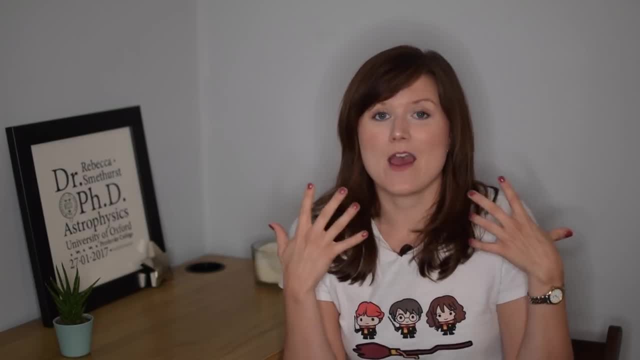 the binary star 70 Ophiuchi. What he'd been doing was observing the positions of the stars in this binary system as they orbited around each other, And he said their positions couldn't be explained if they were the only two bodies in this system. There had to be some unseen body aka a planet. 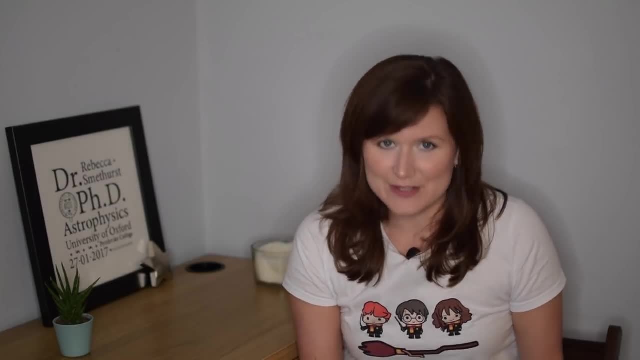 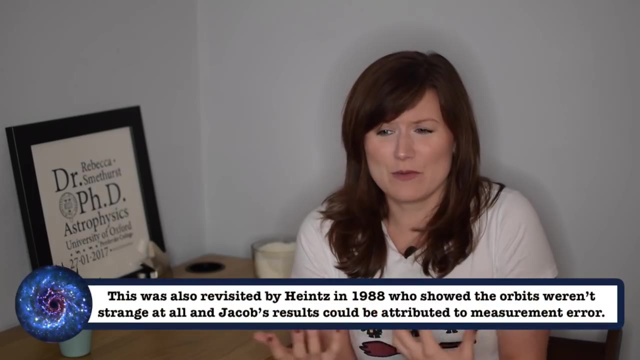 that was there, disturbing their orbits and giving them these weird positions. But that was disproven in 1899 by Forrest Ray Moulton, who pointed out that if you actually did the mathematics, such a planet would have a constant number of stars. And that's what we're going to talk about today. 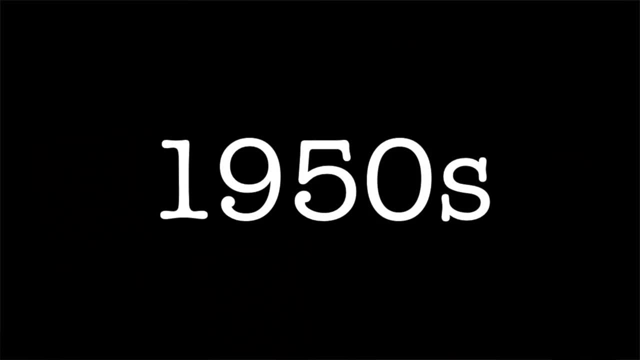 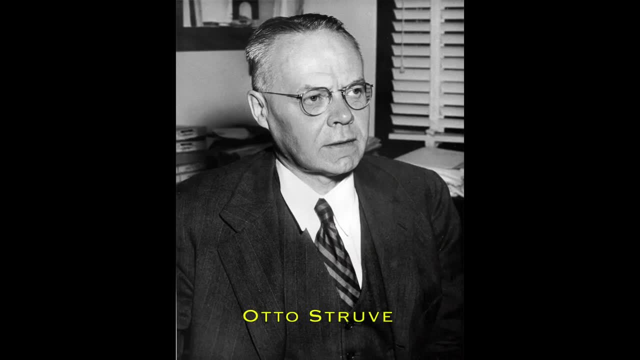 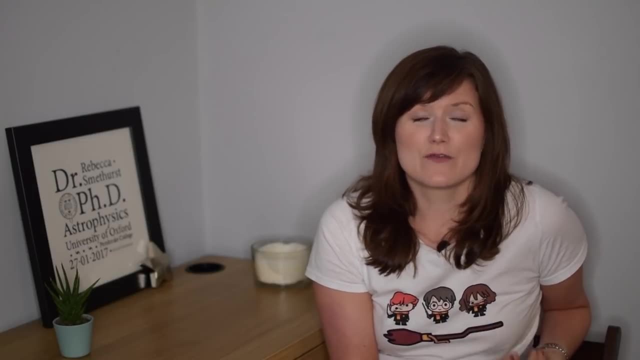 The field of exoplanets, though, had to wait until 1952 for another big leap forward. That came from Otto Struve, a Russian-born American astronomer who really was one of the most high profile astronomers of the 20th century, And he turned this search for exoplanets from. 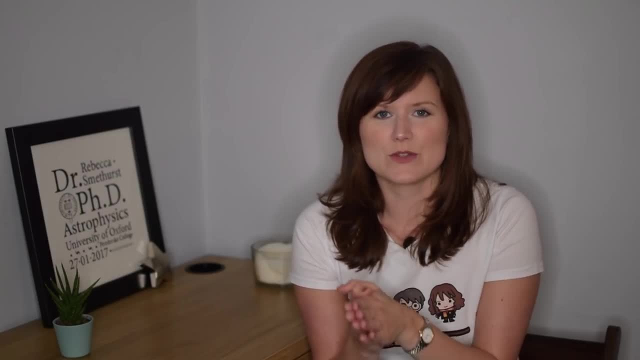 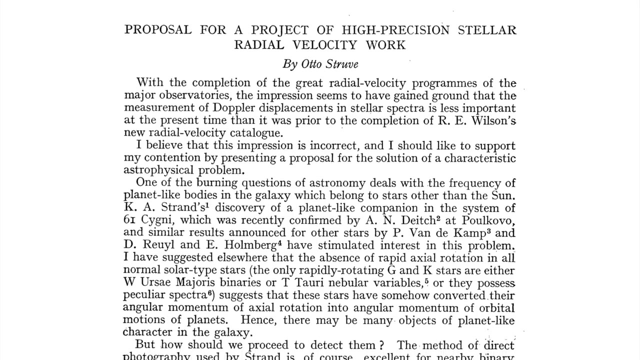 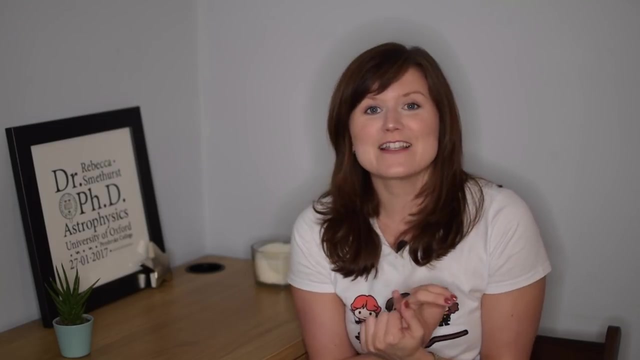 sort of a sci-fi type of thing to really something that was more realistic. He published a paper that said: okay, if we are seriously going to search for planets outside our solar system, then we have to come up with scientific methods for doing so. And well, here's two we could try, And the first one he suggested was that we study the brightness. 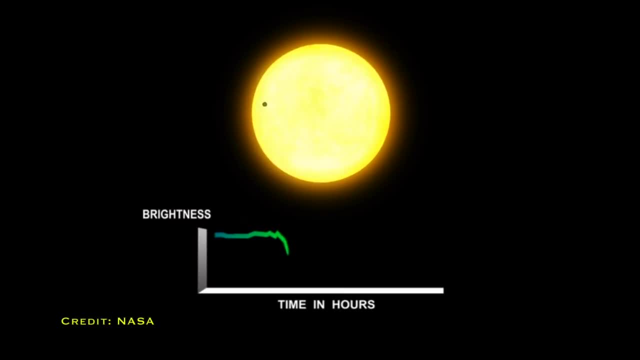 of stars and we see if the brightness dips periodically. If the brightness dips, then you can say: well, perhaps a planet has actually passed in front of that star and we've recorded every 10 days or every 10 years perhaps. And if we see that same brightness dipping, 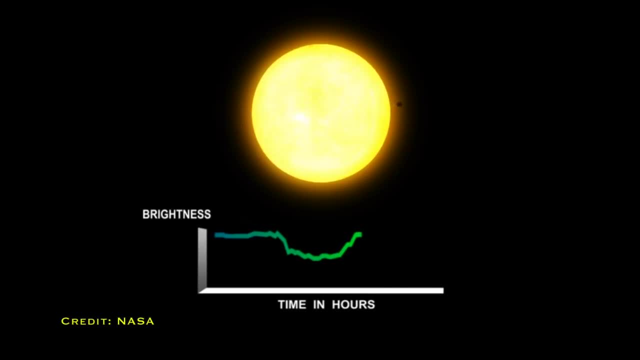 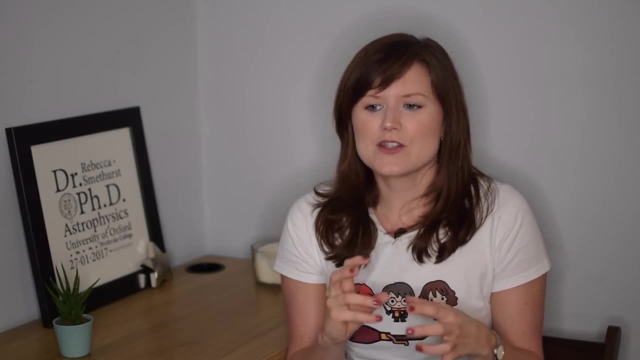 on that exact same repeatable time scale, then we can be sure that what that we're seeing there is a planet orbiting its star. The other method that he suggested would also work was looking for changes in a star's radial velocity. So if you imagine a planet orbiting a star, 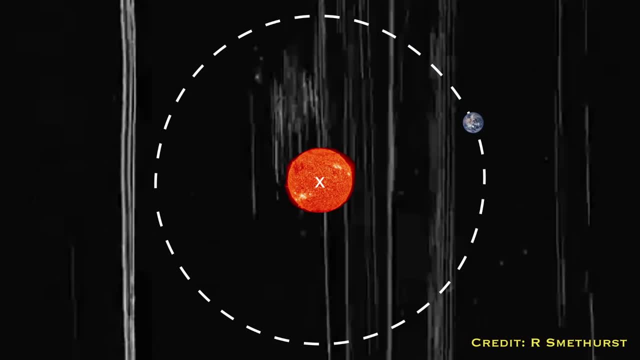 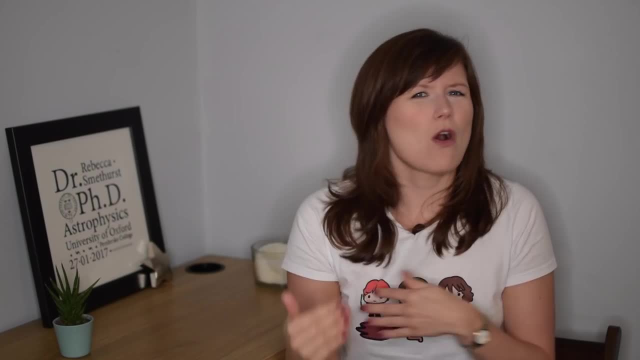 you sort of tend to imagine the star being in a fixed position and the planet orbiting around the very center of the system, which is in the very center of the star. The thing is that's not quite true. If you imagine starting with two objects. 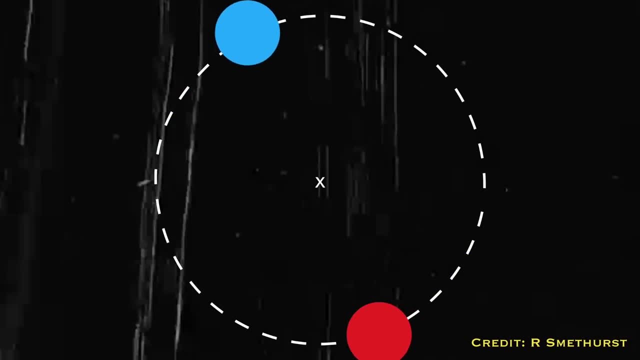 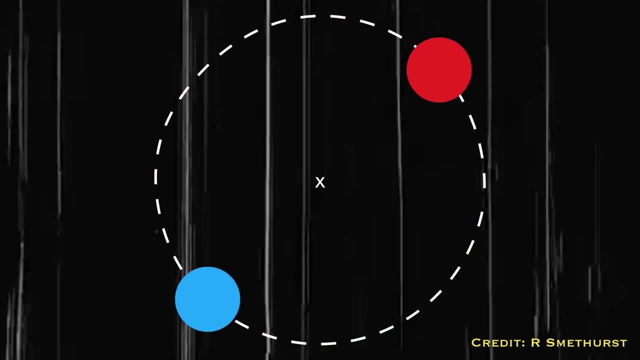 that are the same mass and they're orbiting each other, then they'll orbit the very center of mass between them, which will be halfway between them, and they'll orbit like a binary star system does. If you make one mass then much smaller, then that center of mass will shift towards. 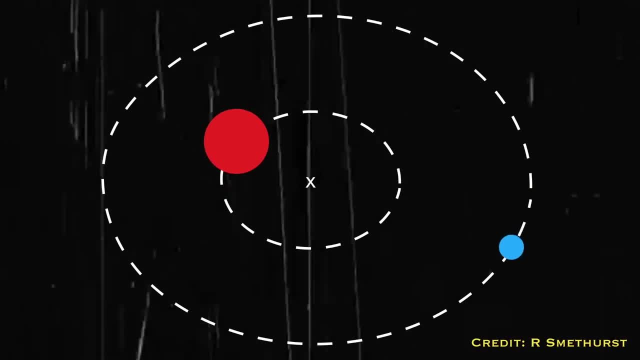 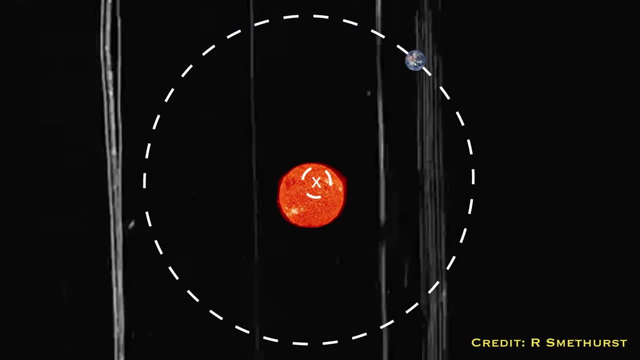 the larger object And if you keep making one of them smaller and smaller, eventually that center of mass will shift so that it's inside one of the objects. And that's what happens when a planet's going around a star. The center of mass is inside the star, but it's not exactly. 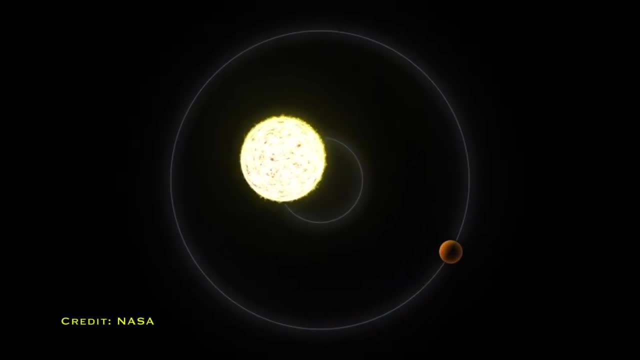 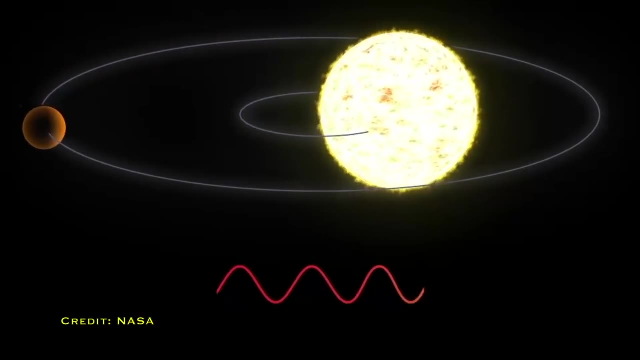 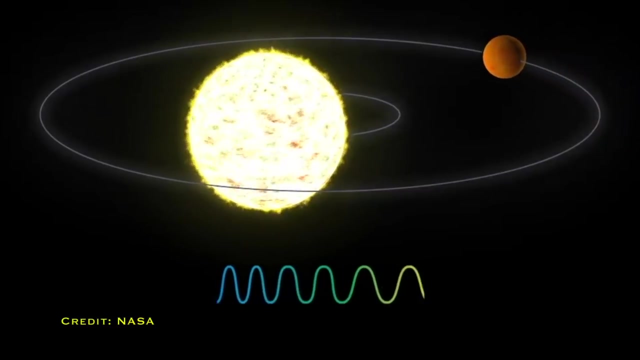 in the center, and so the star itself is orbiting around a point in its middle, and so what that appears to us is like the stars kind of wobbling on the sky, and we can detect that wobble in the light that the star is giving out, because at some points the star will be wobbling towards us and at 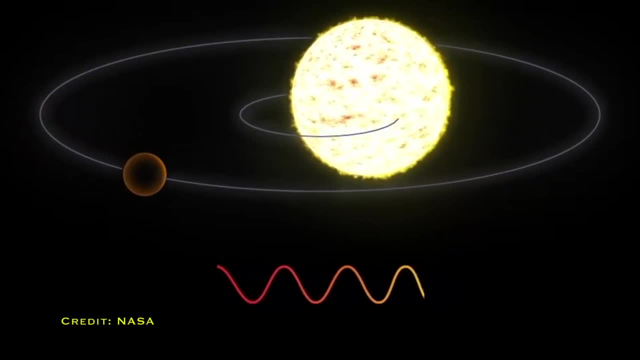 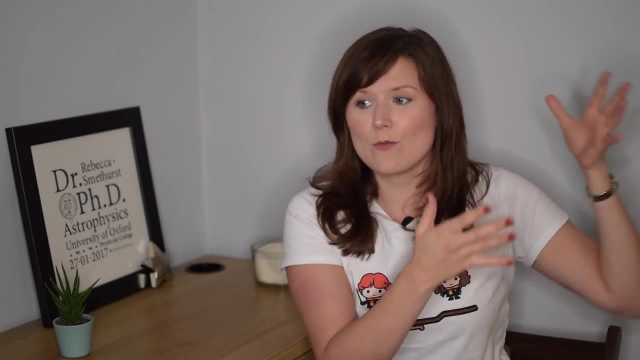 some point it'll be wobbling away from us and just like with a Doppler shift with sound, when an ambulance, you know, comes screaming past us, when it's coming towards us, the pitch of the ambulance gets higher, and when it's moving away from us, the pitch of the ambulance gets much lower. That's. 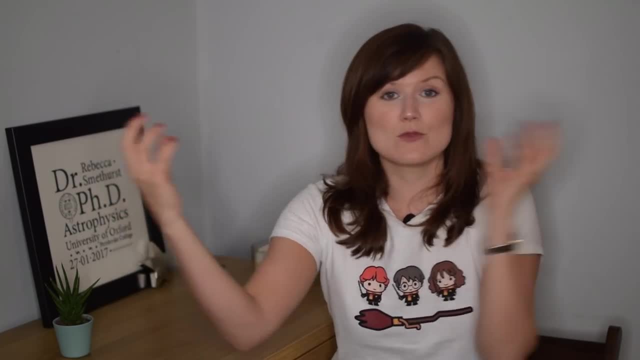 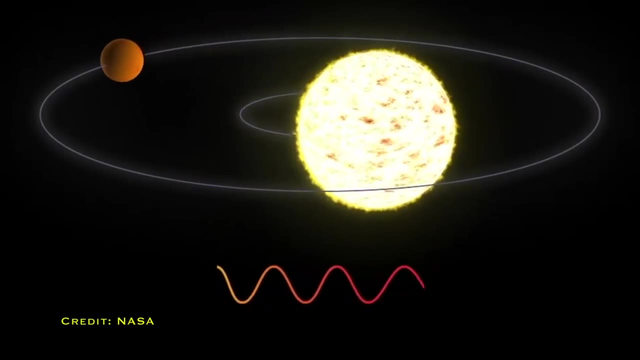 because the wave is being literally squashed and stretched by the ambulance moving towards and away from us. The same thing happens to the light of the star that it's giving off, and so we call that a red shift when it's moving away from us and a blue shift when it's coming towards us. And by 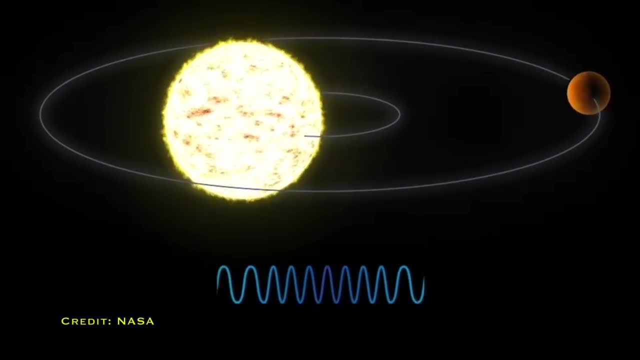 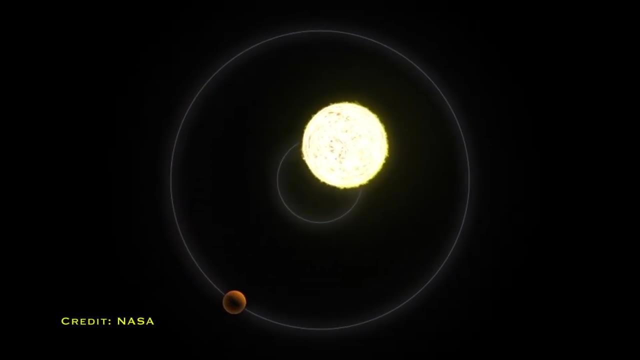 detecting that we can detect how fast the star is actually moving around that little center and then you can determine how big the planet is orbiting around it by how much it shifted that center by. The problem was that in the 1950s the technology was nowhere near good enough to 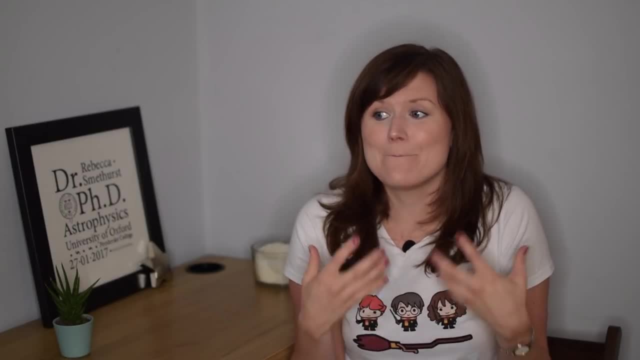 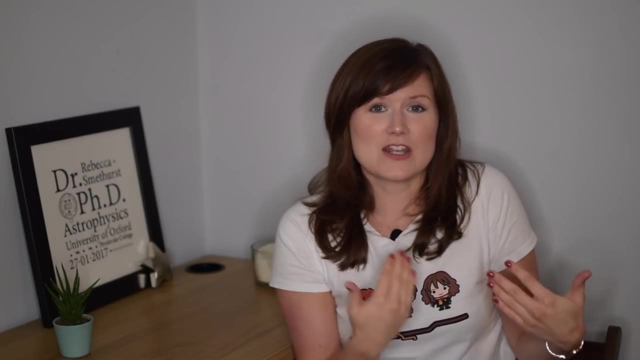 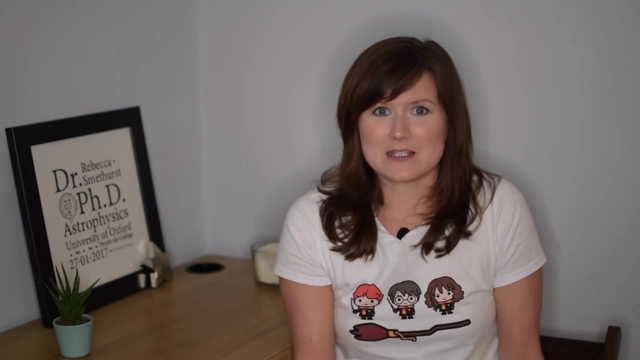 actually detect those shifts. The instruments they were using were giving measurement errors of over a thousand meters per second in a velocity change, whereas if you compare that to the velocity change that Jupiter gives to the sun, it's 12 meters per second and earth is something like 0.1 meters per 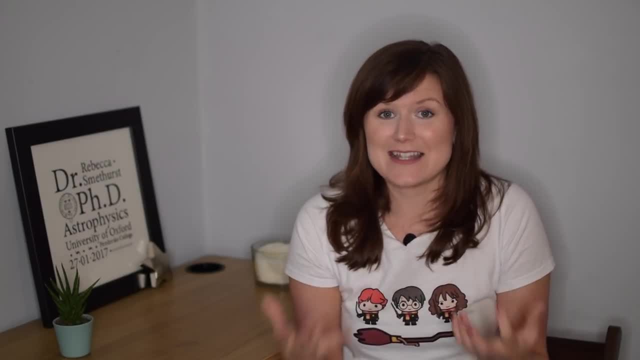 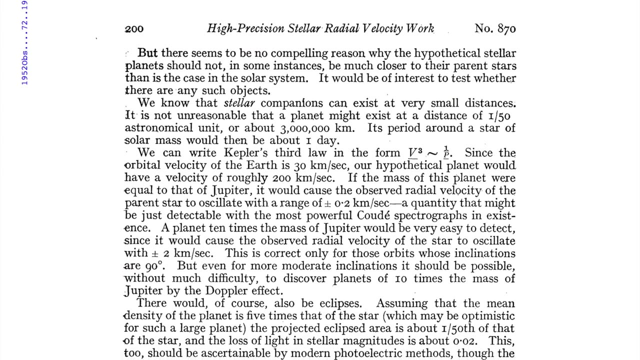 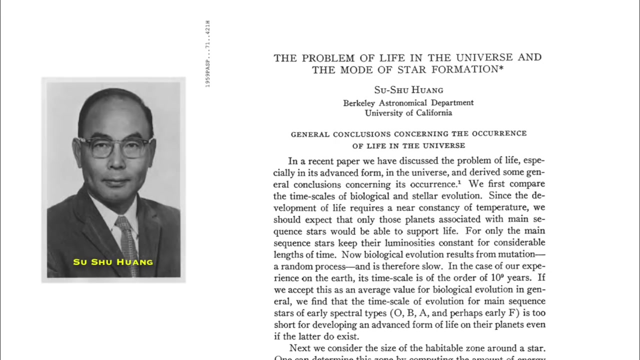 second, so they were nowhere near the level they needed in order to actually detect exoplanets at the time when Otto Struve suggested this method. But that paper did make the prospect of detecting exoplanets much more scientifically realistic and it did get people thinking, so much so that Huang 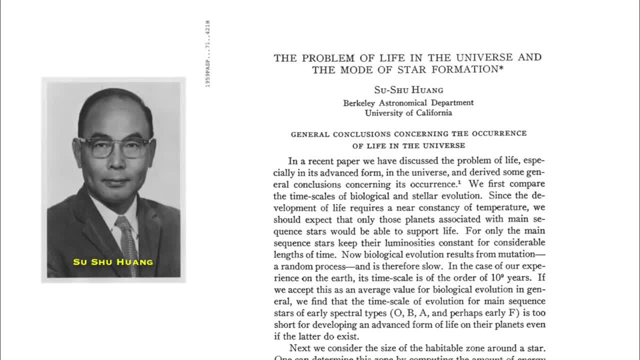 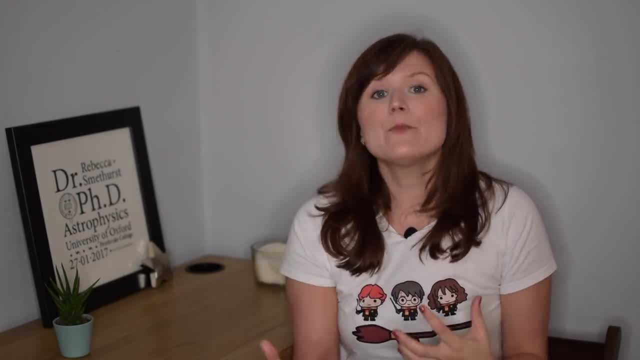 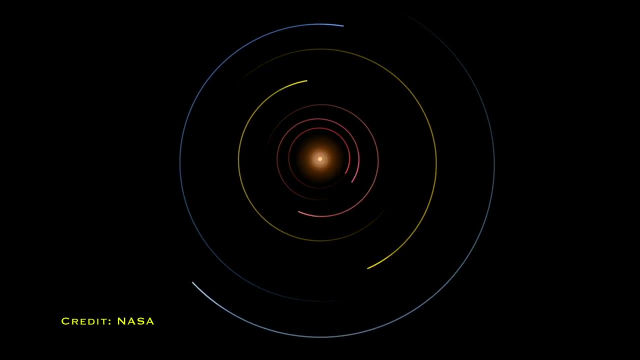 in 1959, published a really famous paper where he introduced the idea of a habitable zone around a star, The region around a star where the temperature on a planet would be between 0 and 100 degrees centigrade, ie a freezing and boiling point of water. It would be the region where you would find liquid water. Note. 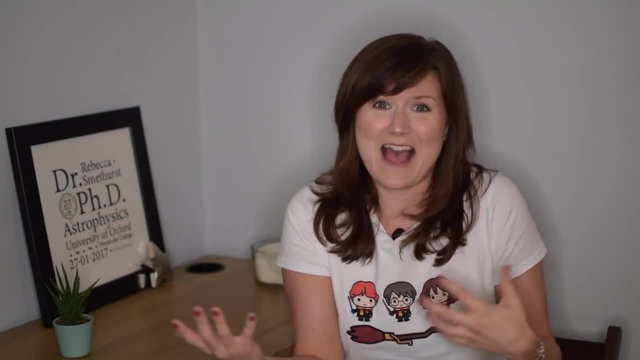 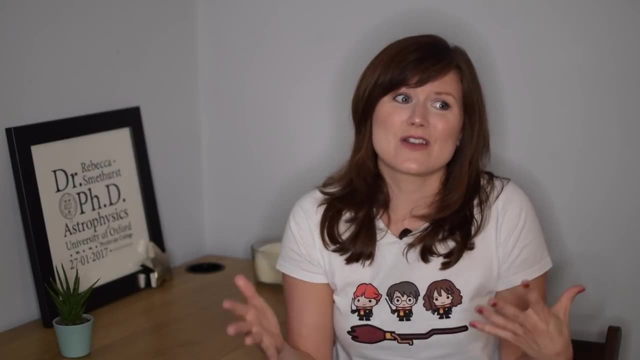 that it doesn't mean that it's habitable to humans, because, well, Mars is in the sun's habitable zone, but it doesn't have an atmosphere that can support human life. it's lost it all to the solar wind and so obviously that's not habitable, but it is a good way of at least characterizing it. So the ideas of the 50s, and presumably the space race in the 60s as well, really spurred people on in this search for exoplanets. so much so that there was a huge flurry of false alarms again, One of the most high profile of them- by Peter van der Kamp in 1963. 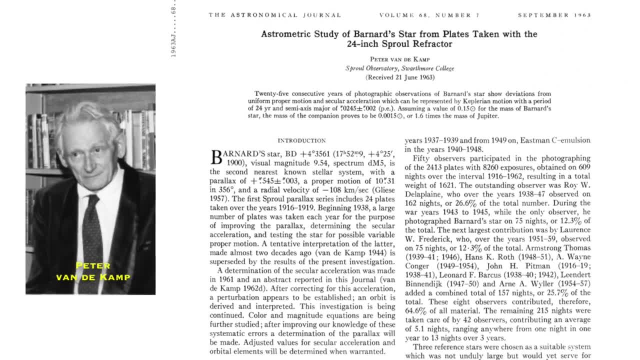 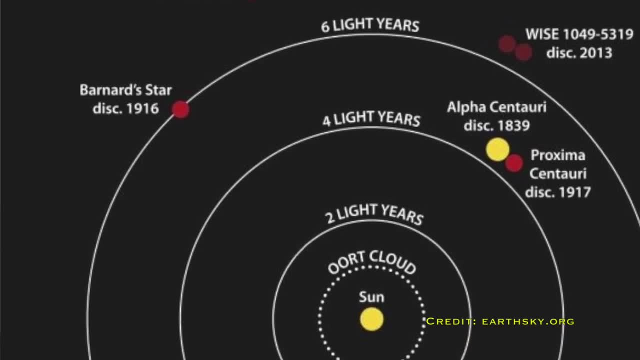 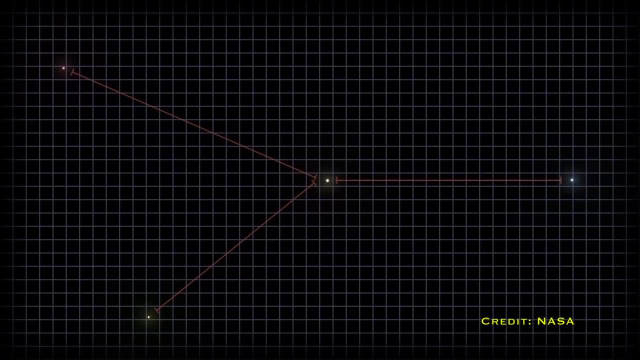 who claimed he discovered a planet around Barnard's star, which is one of the closest stars to the sun. He claimed he detected the star wobbling in its orbit, but not using the redshift like Otto Struve had suggested, but actually by studying the position of the star on the sky- His paper. 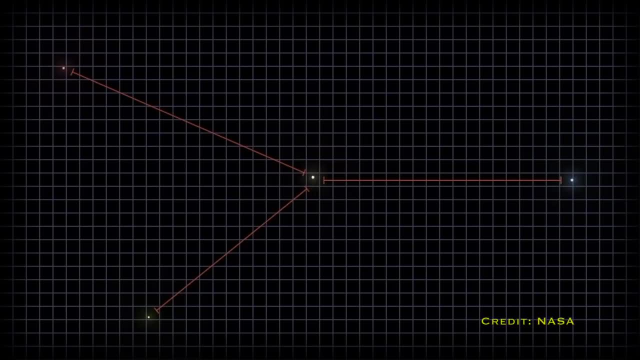 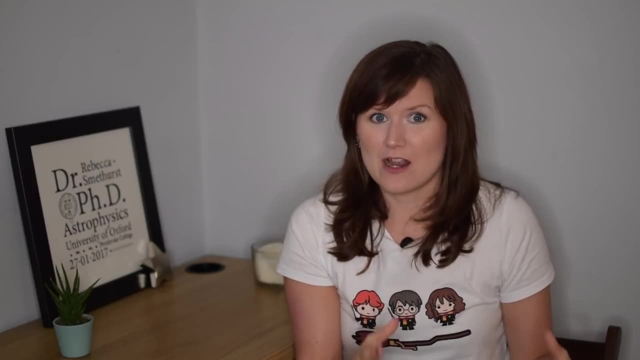 suggested that from the changing positions of Barnard's star to the sun's habitable zone that there was a 1.6 times the mass of Jupiter planet there, orbiting at about 4.4 times the distance of the earth and the sun. He then refined that estimate in 1969 to say: actually, I think 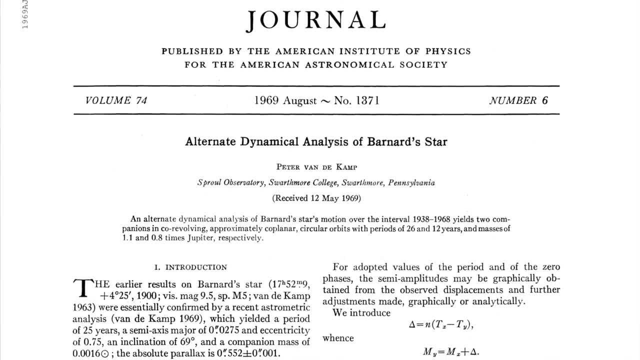 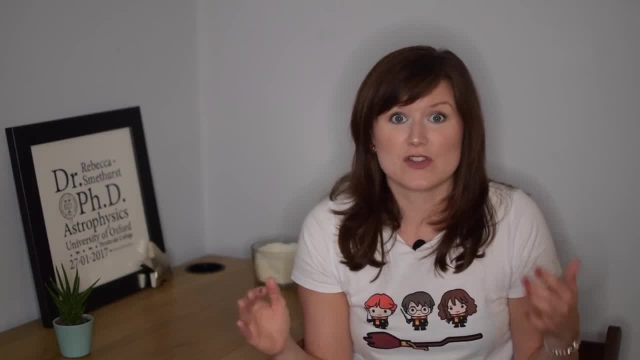 there's two planets: one that's 1.1 times the mass of Jupiter and one that's 0.8 times the mass of Jupiter. The problem was that many astronomers could not reproduce his observations at all, not for want of trying, but they couldn't find these changes in positions that he'd claimed. 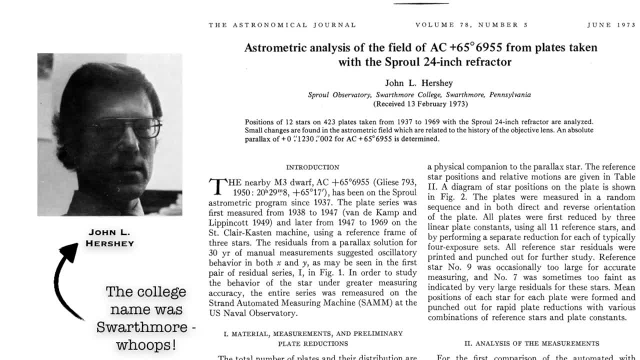 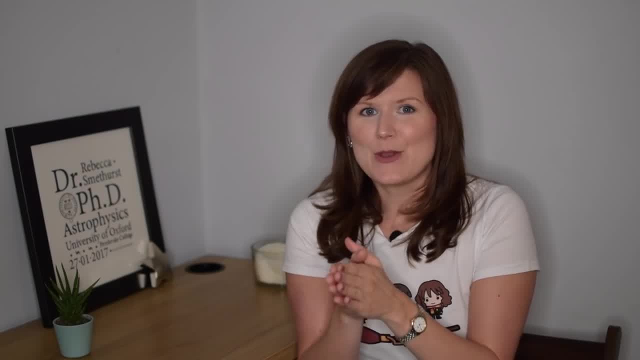 And it actually took until 1974 when Swarthmore showed that the changes in the positions that van der Kamp had actually recorded correlated with the times when the telescope that he'd used had maintenance on it or was recalibrated, And so the changes in the positions in the 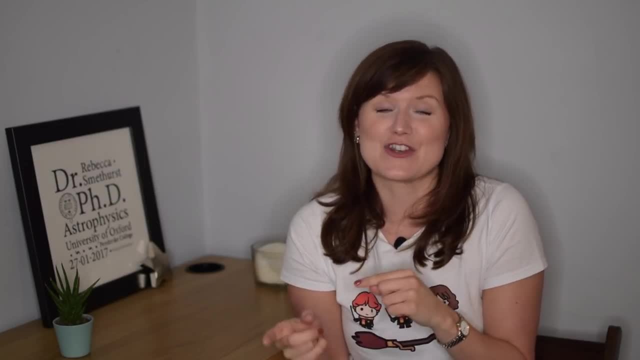 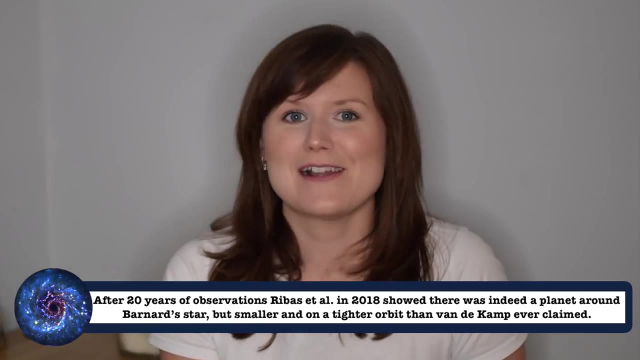 star that he recorded were actually just a change in the position in the telescope. That's how accurate these kind of observations need to be. If you don't account for the fact that your telescope has changed ever so slightly on its mount, then you're going to 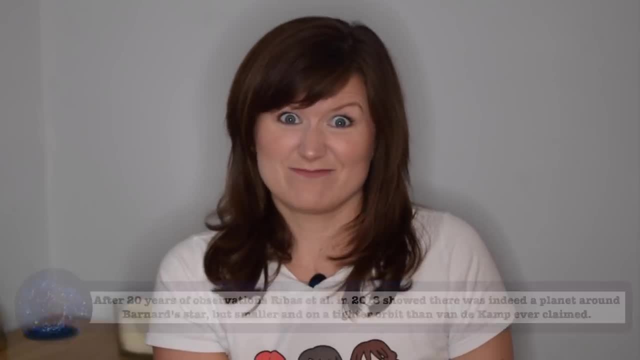 end up with the same kind of observations that you're going to end up with on your telescope: incorrectly assume that there's a planet around a star when there's not. By the 1980s, telescopes had improved leaps and bounds, so much so that Bradford Smith and Richard 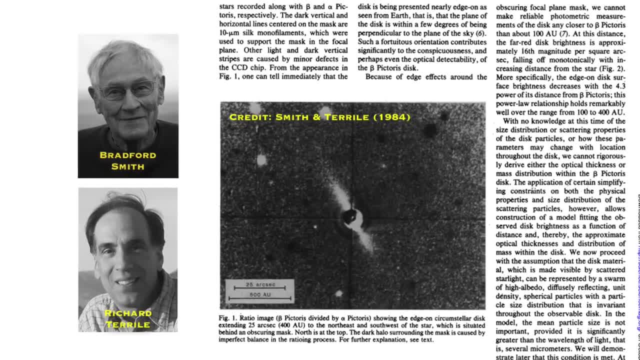 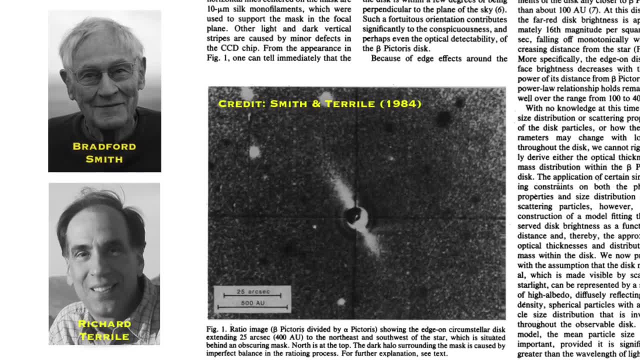 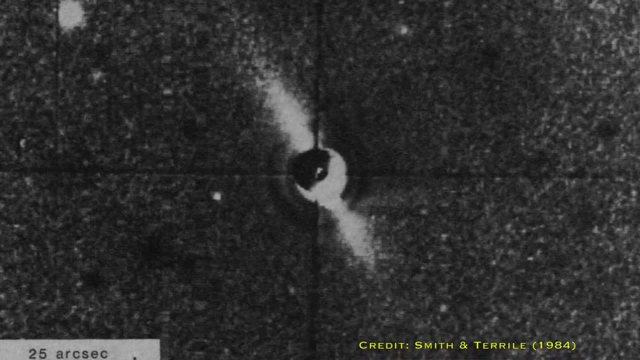 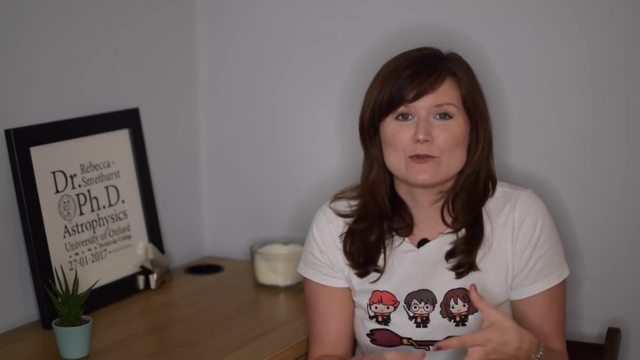 Tyreel actually managed to image material around the star Beta Pictoris. What they'd imaged was sort of a dusty disk surrounding the star, which, from planetary formation models, was expected if you were forming brand new planets around that star. It was the first time any material around a star had been detected in visible light. 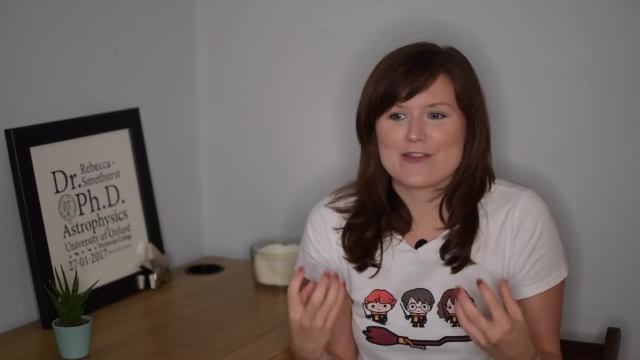 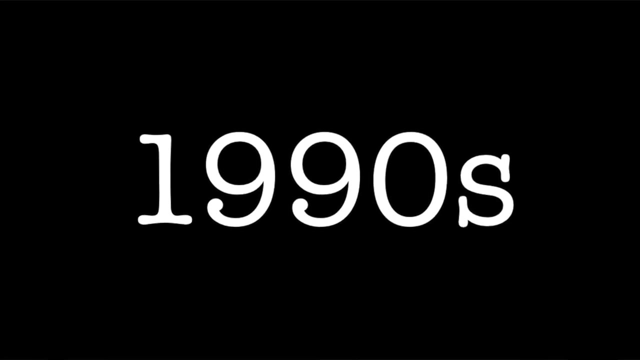 and it really spurred people on again to actually try and find the first fully formed planet around a star. As we head into the 1990s, the first thing I want to mention is that the Hubble Space Telescope was launched in April 1990, a mere month before I came into the. 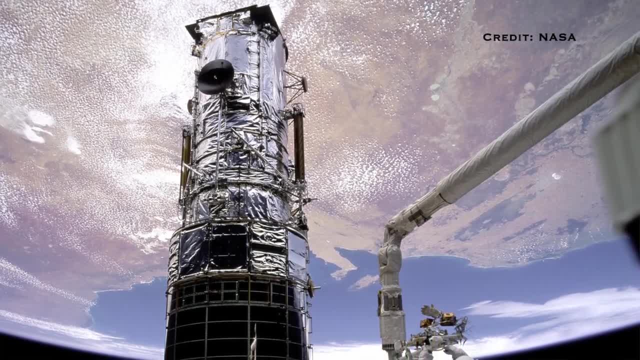 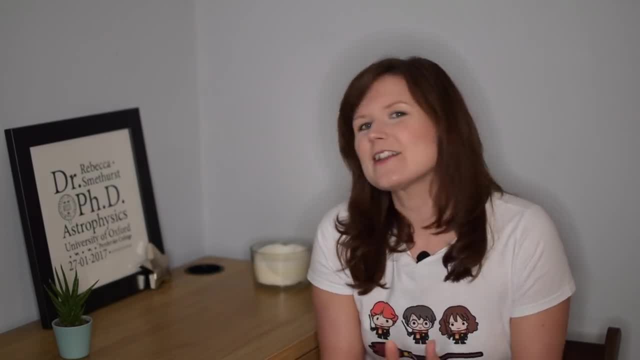 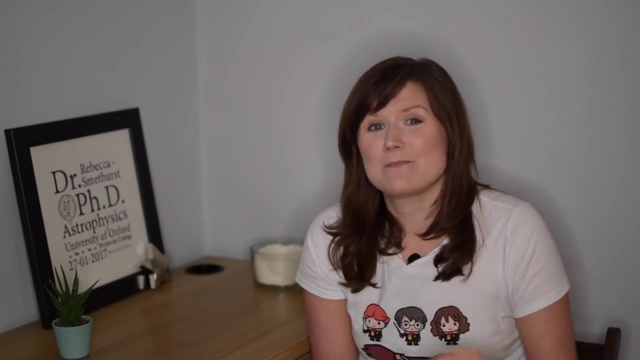 world. After a few minor teething problems with its mirror, it became a telescope that was instrumental in the study of exoplanets. Then, in 1992, the first discovery of a planet finally came, but in the most unexpected of places. It wasn't around a star like the sun. 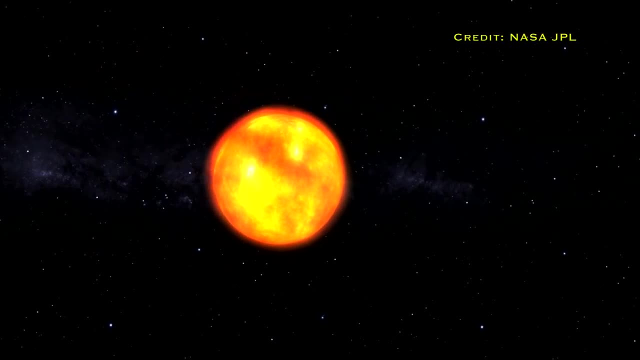 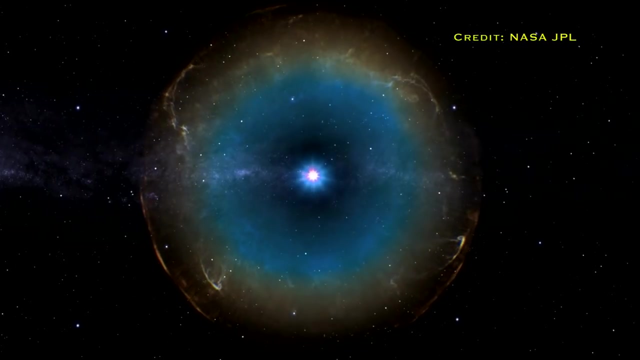 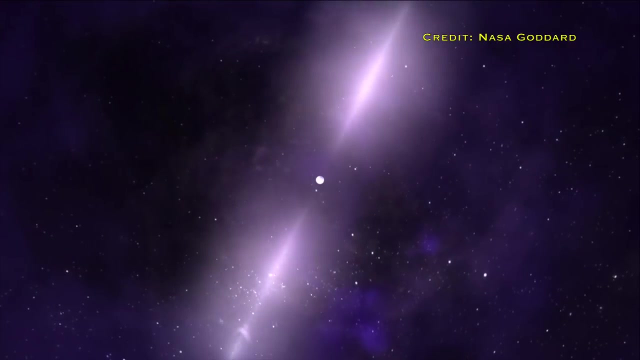 it was around a pulsar. This is something that's formed at the end of a star's life: a massive star that's gone, supernova, and left over this remnant of a neutron star that's spinning and giving off radio waves, So much so that we detect them as pulses of radio waves on earth that you can. 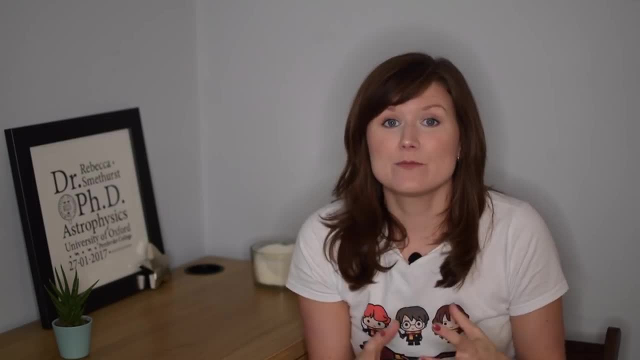 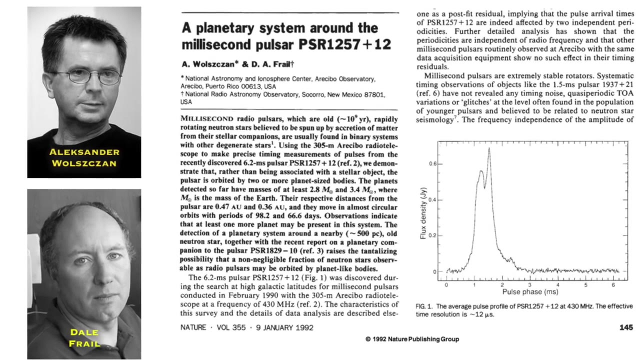 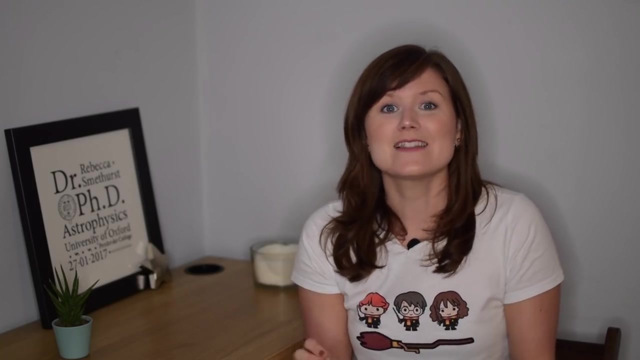 literally set your watch to. They are incredibly precise and it was Alexander Wolkazan and Dale Frail that showed that the arrival of the pulses from pulsar 1257 plus 12 were off ever so slightly and that could only be explained by the presence of two planets orbiting that pulsar. That, as they 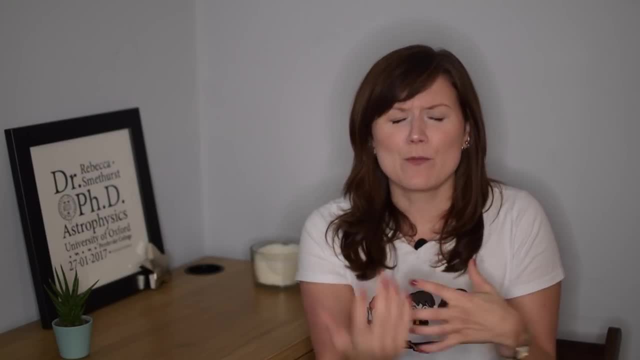 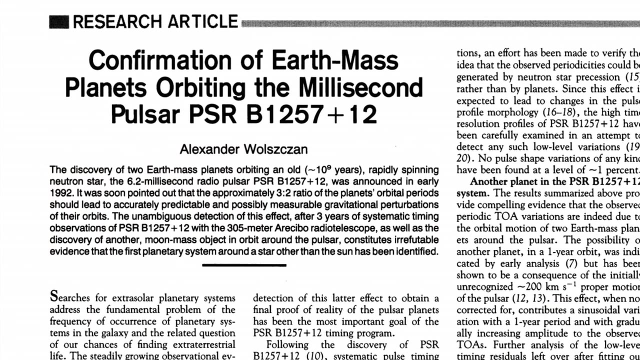 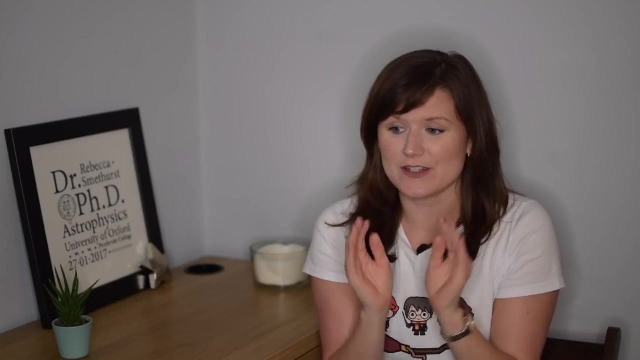 orbited it, they would actually delay The radio pulses arriving to us on earth. They even did follow-up observations and released another paper in 1994 to say actually the two-planet model wasn't quite right and we actually need three planets to describe this system. I cannot stress enough how much of a 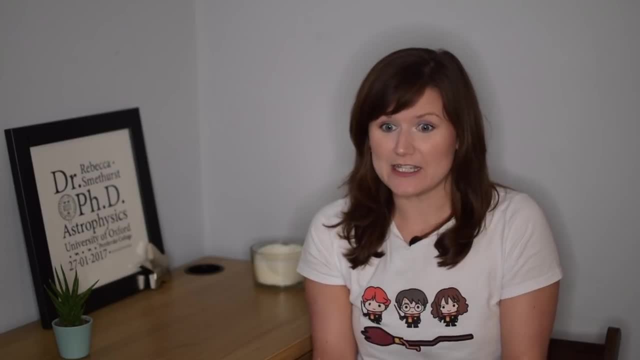 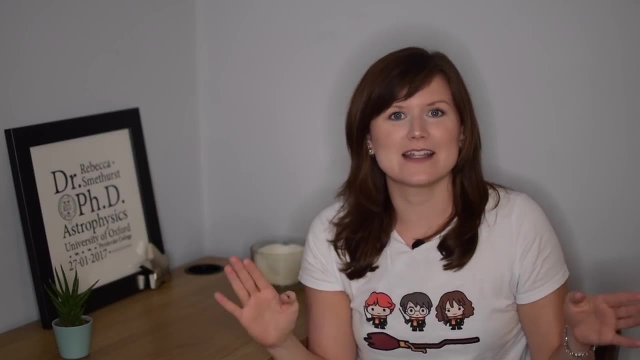 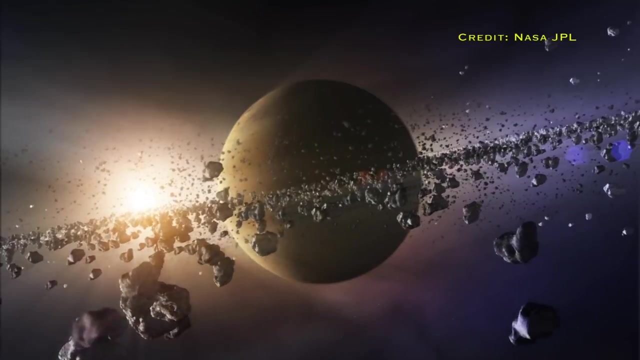 surprise this discovery was to the astronomy community. Nobody expected this. Everyone literally had to rethink their entire view of how planets formed. You know, originally people thought that they formed as a star, formed from the leftovers of whatever didn't form the star. but to find three planets that were only slightly bigger than the earth orbiting around. a pulsar. that would mean either the planets had to fully survive the supernova that formed the pulsar in the first place, so perhaps they were big gas giants like Jupiter that had all of that gas strip just leaving the core around the pulsar, or perhaps you've had like a secondary. stage of planet formation where the supernovas happen, destroyed everything around it but then left all this debris where you've had this second round of planet formation around the pulsar. So it wasn't necessarily the result that people wanted, but it definitely gave people a lot to think about. 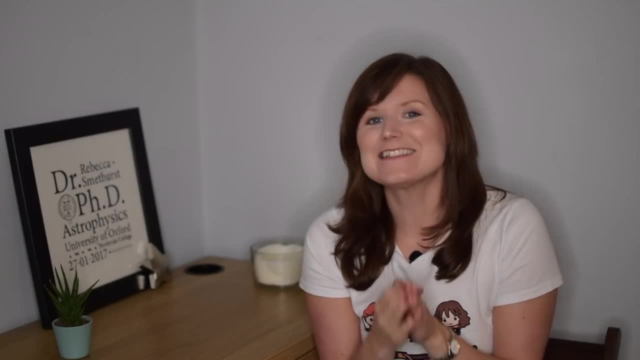 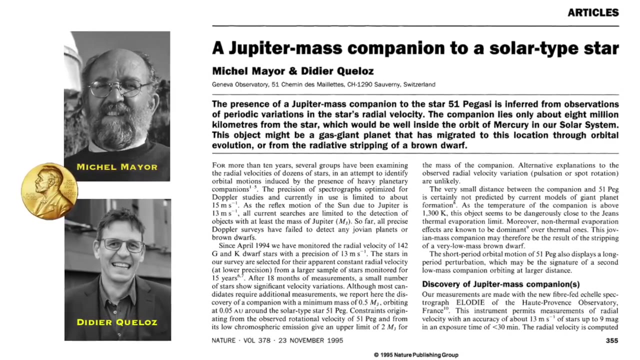 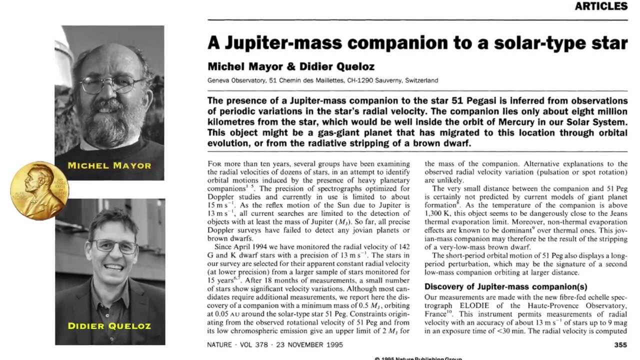 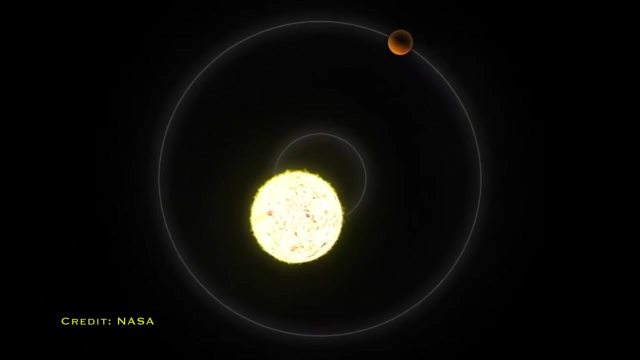 It was then, finally, in October of 1995, that Michael Mayor and Didier Queloz discovered the first exoplanet around a normal star. In fact, it was a star that was just like the sun. To do that, Didier and Mayor studied 142 different stars for over a year, watching for those little blue and red shifts. 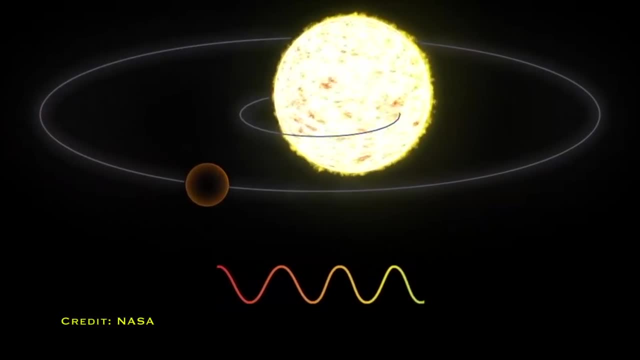 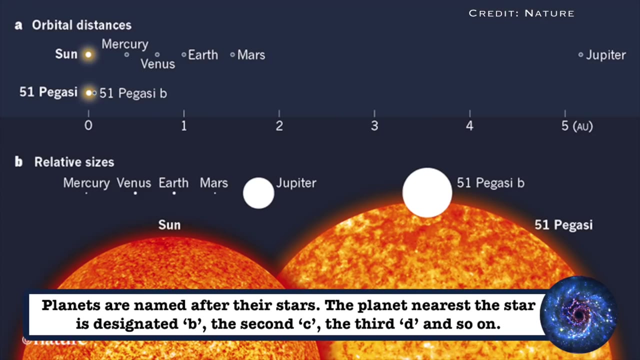 that would suggest that there's a planet going around it, and finally found this one, 51 Pegasi b, But it was a planet that was two times the mass of Jupiter and it orbited only five percent of the distance between it and Jupiter. It was a planet that was two times the mass of Jupiter and it orbited only five percent of the distance between it and Jupiter. 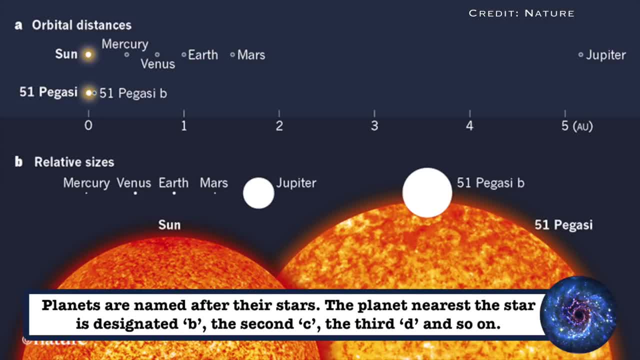 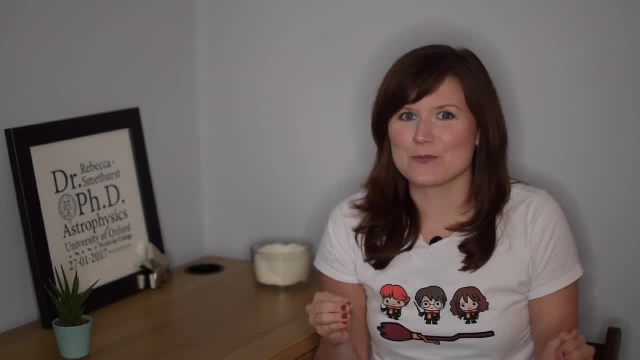 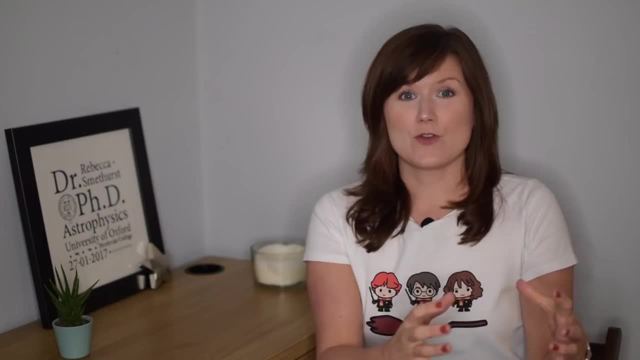 the earth and the sun that would be inside the orbit of Mercury, in our own solar system. Once again, though, the astronomy community was absolutely stumped by this result: It was a Jupiter inside the orbit of Mercury. No one had ever considered that before, because all planetary formation models have been based on well, the one example we had to go off. 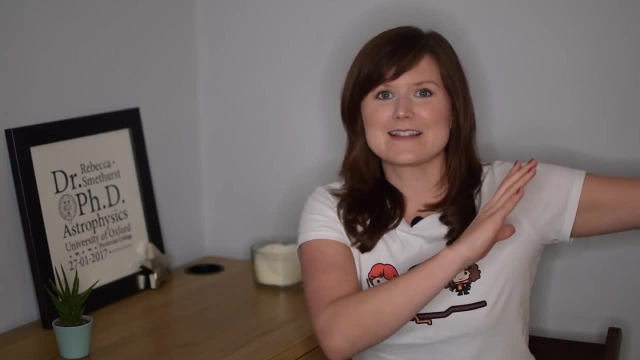 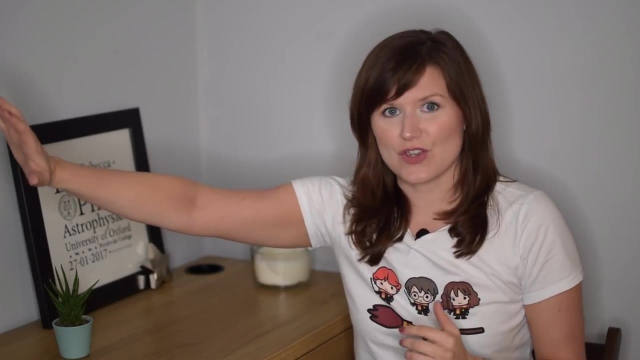 which was the solar system where we find rocky planets in towards the sun and the big gap and the big gas, giant things up to the size of Jupiter way out on the outskirts. People then started to consider the idea of planetary migration where you could form something. like Jupiter, from the ices and the gas that were found well out from a star, and then it could actually migrate and move inwards so that its orbit was ever smaller and smaller. Even now we actually think that that was supposed to happen in our solar system, but Jupiter was sort of held back. 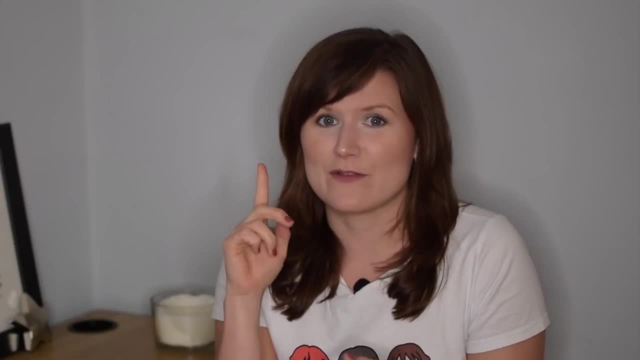 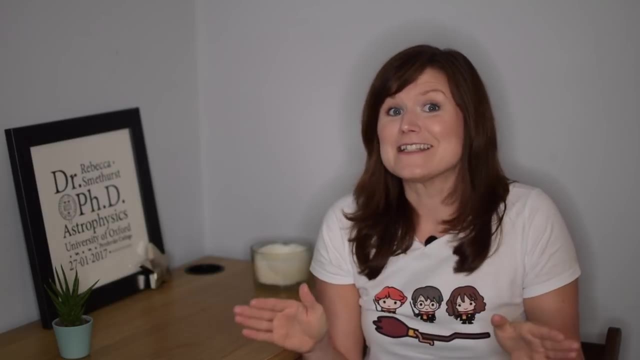 from doing that by the presence of Saturn. so we should all be very thankful for Saturn. It's why it's my favourite planet. But after this momentous discovery by Didier and Mayol, the floodgates really did open on the field of exoplanets, In particular, Butler, Marcy Williams, Hauser and 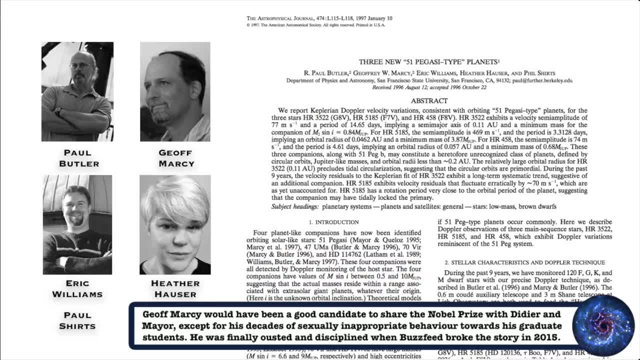 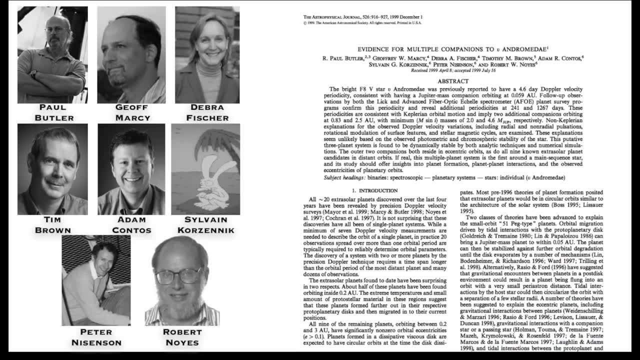 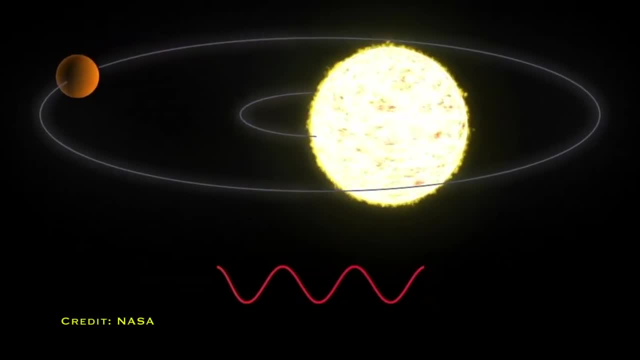 Schertz found a planet around Upsilon Andromeda in 1997 and then in 1999 with the help of a couple of other colleagues, including Fischer, Kongos, Keresnick, Nisar and others. Nissen and Noyes realised that the observations of these little blue and red shifts of the star 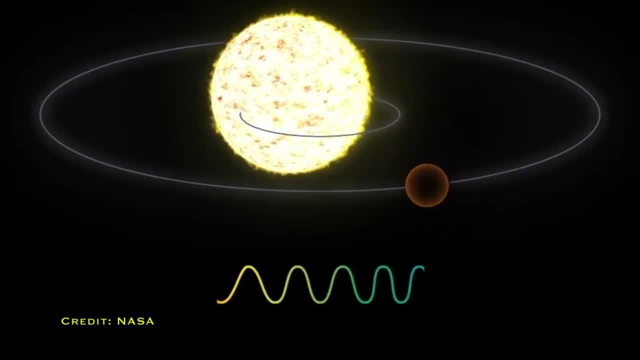 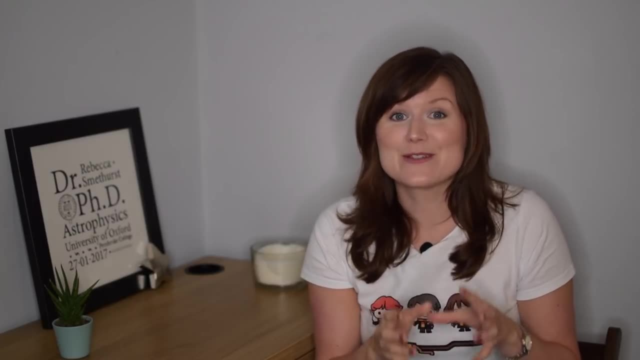 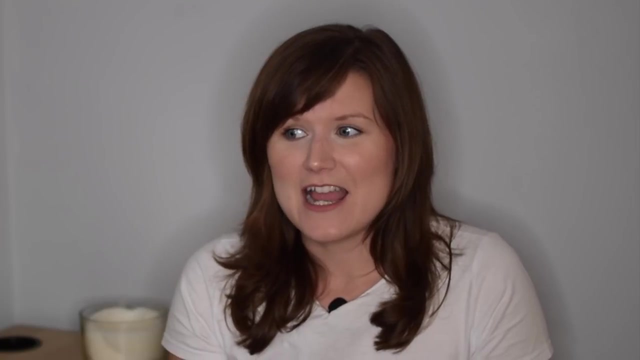 Upsilon Andromeda. this radial velocity measurement didn't match a one planet model. They needed three planets in orbit around that star to be able to explain what they were seeing. This was the first multi-exoplanet system found and it showed that the solar system wasn't unique in the universe. 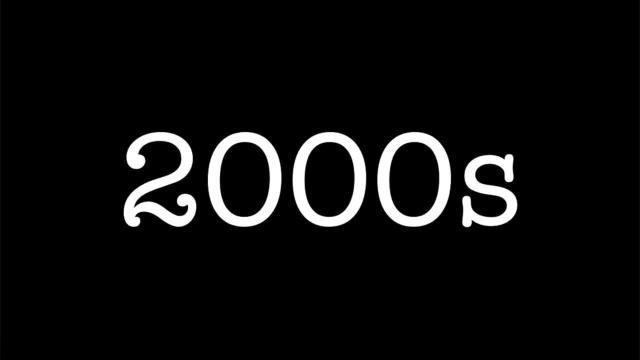 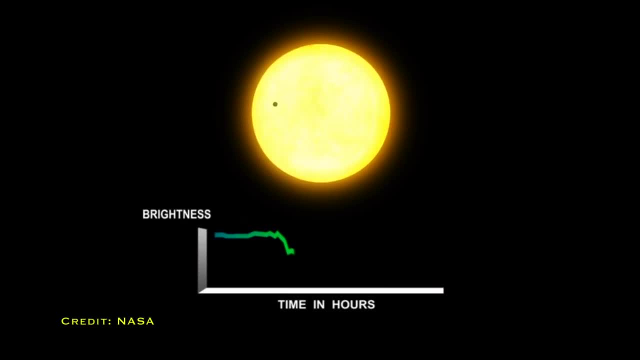 at all. But then in the 2000s, which was really a decade of firsts and in particular the very first planet that was detected using the transit method. Now it'd already been found using the radial velocity method, where you look for those blue and red shifts of the star. but that meant that people knew when to look for. 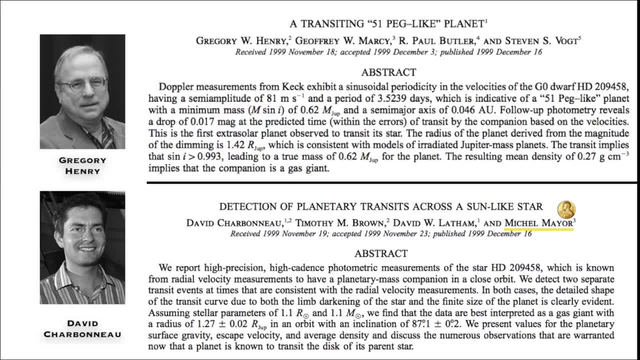 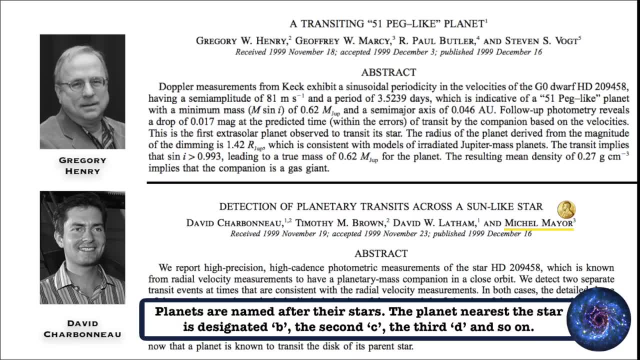 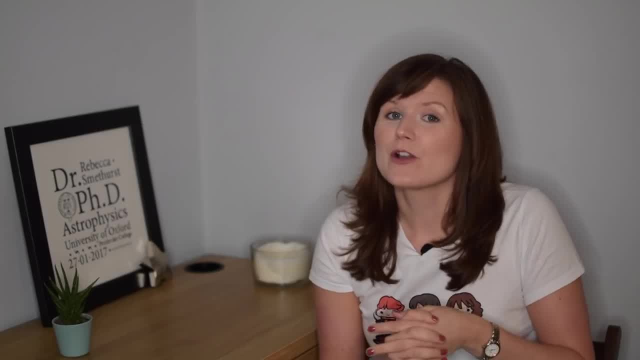 the transit, and so two groups did that independently and published at the same time and announced that they had observed transits of HD 209458. Meaning that the planet around it was HD 209458b. The observant among you will notice that you're. 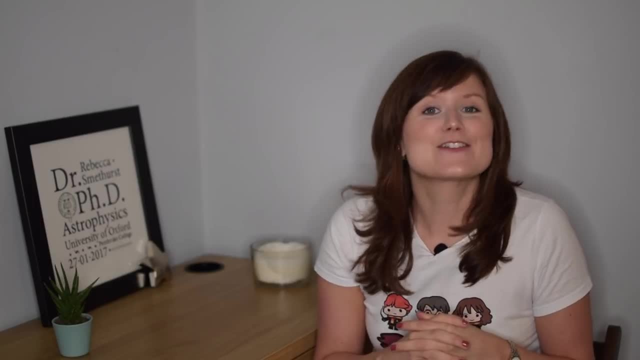 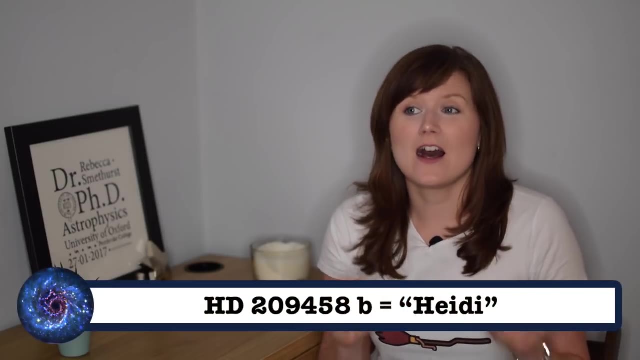 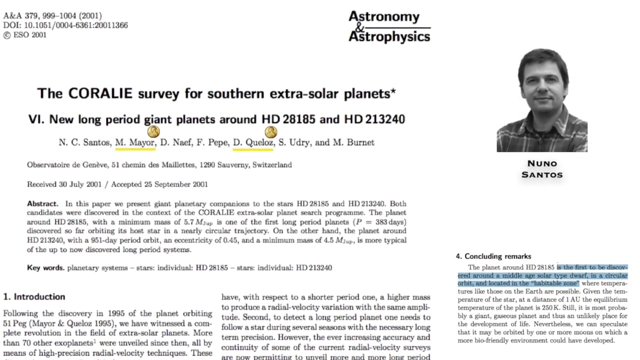 going to see that planet popping up a lot in the next couple of results. so just to make it clear how many firsts that this planet is involved with, I'm going to nickname it Heidi, as in HD, Heidi. Before we get to Heidi, though, in 2001, Nuno Santos and collaborators found the very first planet in the habitable zone around a star. 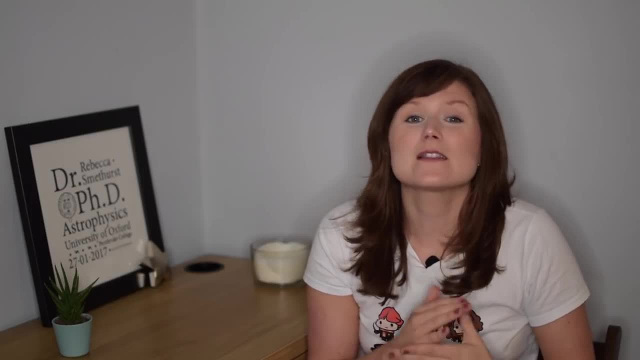 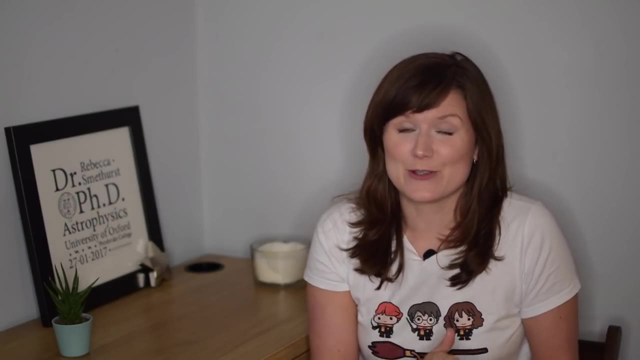 In 2001,, Nuno Santos and collaborators found the very first planet in the habitable zone around a star. It's 5.7 times the mass of Jupiter, so it's not exactly earth-like under any definition, but it is still in the habitable zone, which was a major advancement for the field of exoplanets. 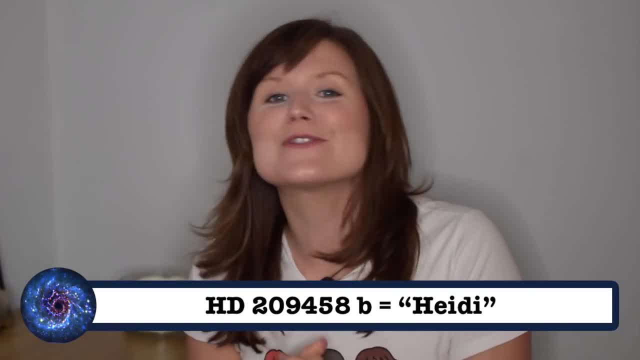 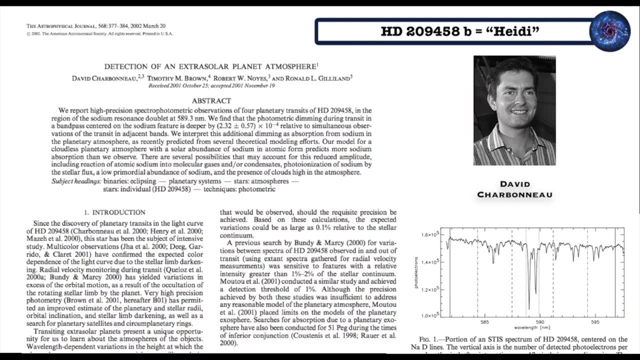 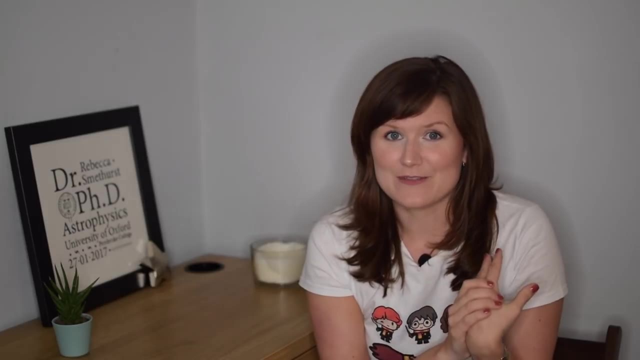 And now the golden age of our friend Heidi HD 209458b. In 2002, Charbonneau and collaborators managed to detect sodium in the atmosphere of Heidi ie in the light that had passed from the star and through the atmosphere on its way to earth, and it became the first exoplanet ever to have its 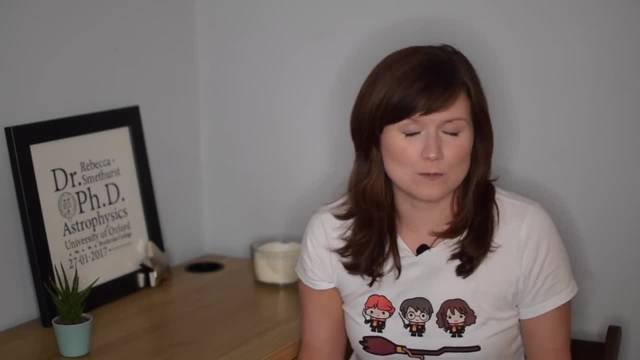 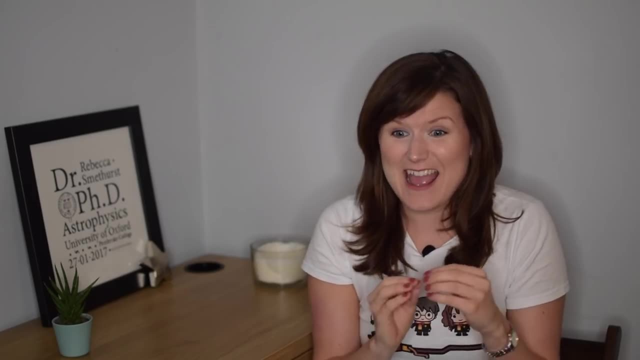 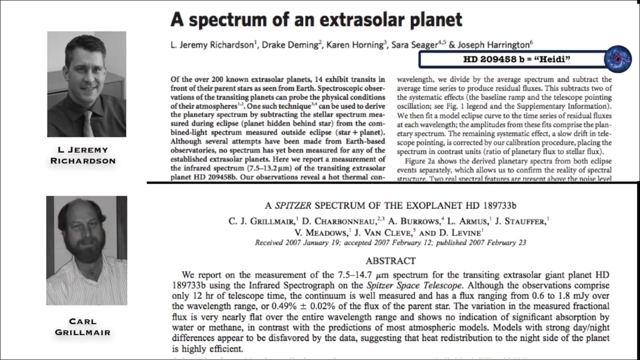 atmosphere characterized in some way or form. In 2005,, Deming and collaborators then managed to isolate the light from Heidi and it became the first exoplanet ever to have radiation specifically from the exoplanet detected In 2007,. two independent groups, one led by Richardson and 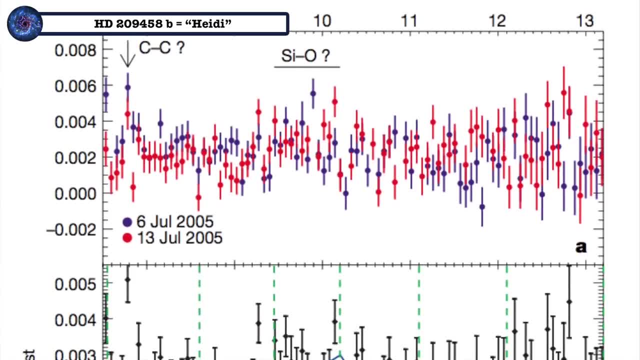 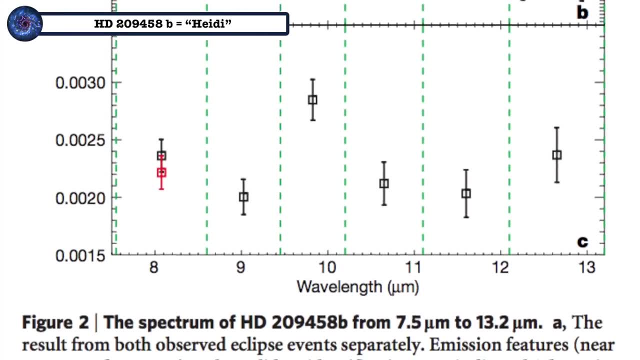 one led by Grillmeier, then managed to isolate the light from Heidi, and then managed to isolate the light from Heidi from Heidi, split it through a prism and produced the very first spectrum of the atmosphere of an exoplanet. And once those two groups had shown that was possible, speculation ran rife through. 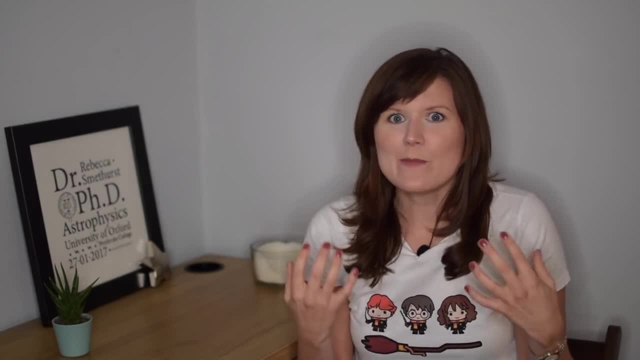 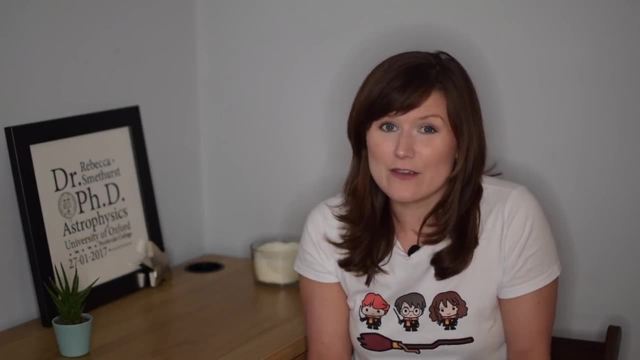 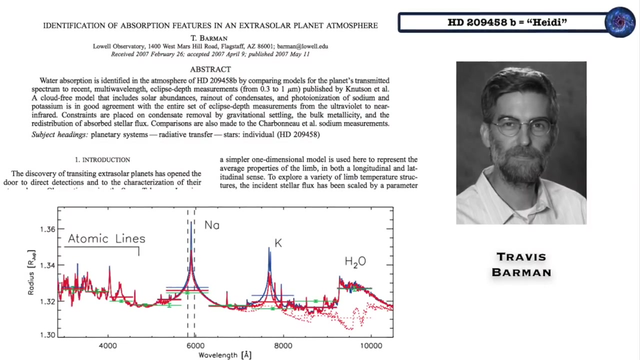 the community of what we'd do with that method. Would we be able to detect water, oxygen, ozone, carbon dioxide- the markers of life on a planet- using that method? An excitement which was only fueled further later in 2007 by Barman, who then managed to take a spectra of Heidi's light. 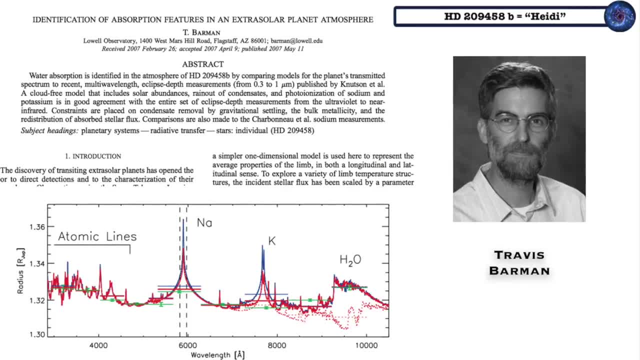 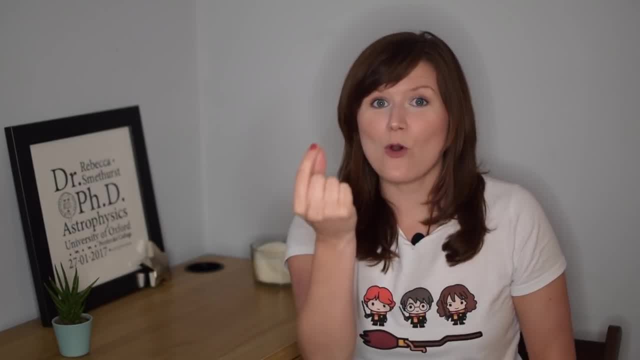 and actually say I've detected absorption by water vapor in the atmosphere, ie the light on the way from the star through the planet's atmosphere was absorbed by water at a very, very specific wavelength that we've seen here on Earth in the lab as well, And they managed to. detect that dip at that wavelength. And so Heidi became the first exoplanet to have water vapor. And so Heidi became the first exoplanet to have water vapor. And so Heidi became the first, the first exoplanet to have water vapor. And so Heidi became the first exoplanet to have water. 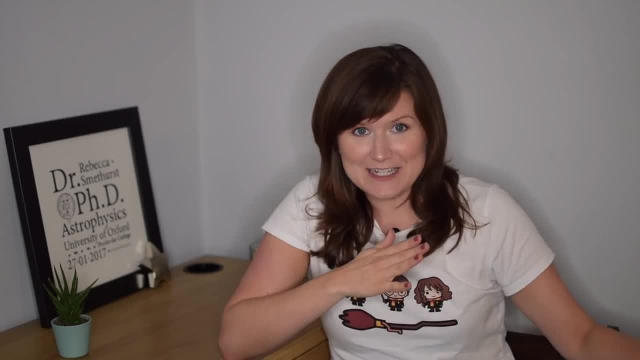 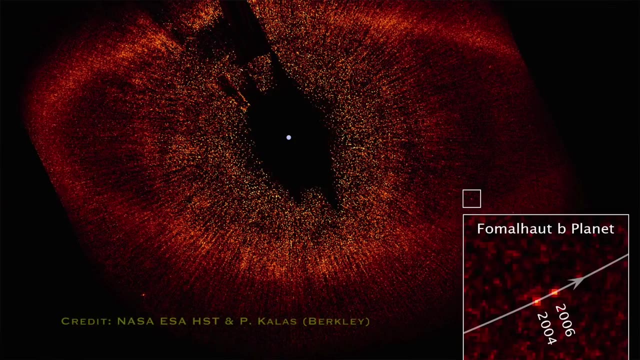 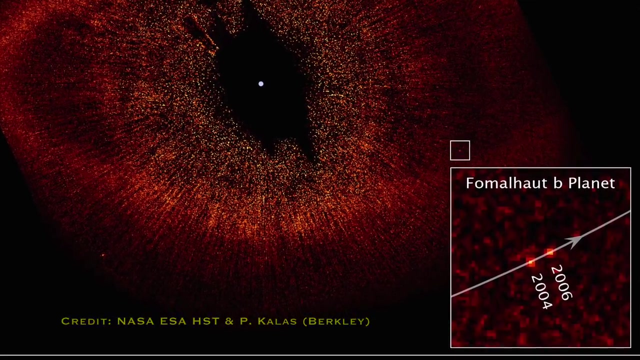 vapor detected in its atmosphere. Okay so, Heidi, hysteria aside, in 2009,, despite all of these detections of exoplanets, we finally had the first image, a direct image of an exoplanet around another star. This was a group effort led by Paul Callas, and it was of the planet Formholt b, a planet 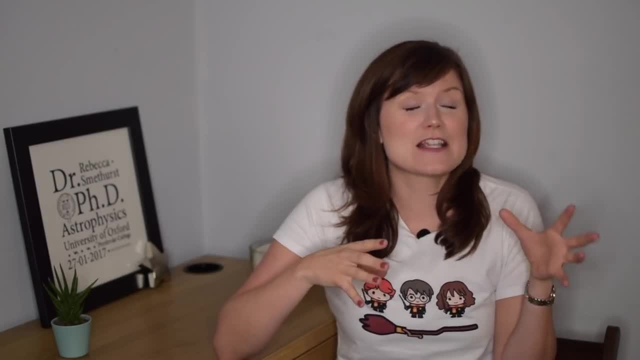 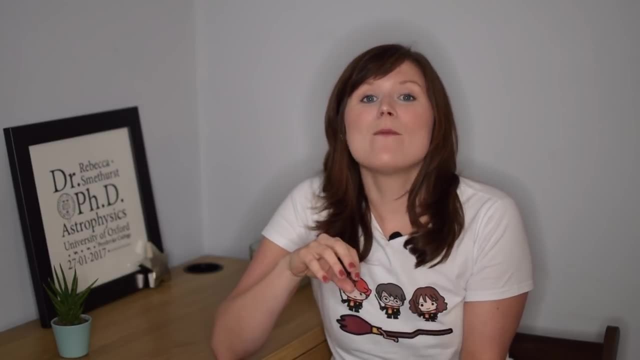 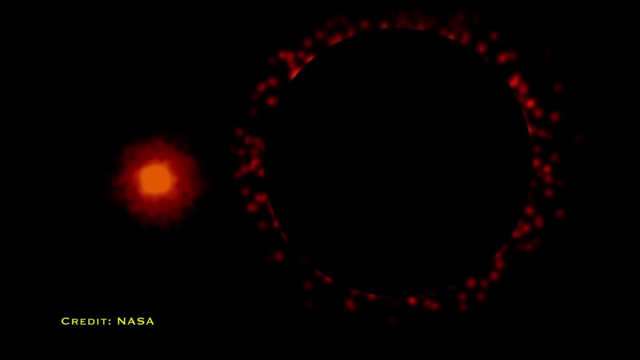 119 times further out than the earth is from the sun- that is three times the mass of Jupiter- And to detect it they needed the Hubble Space Telescope to do that, And what they did was they put a mask on the detector to block out all of the light from the central star, And they took an image in 2004. 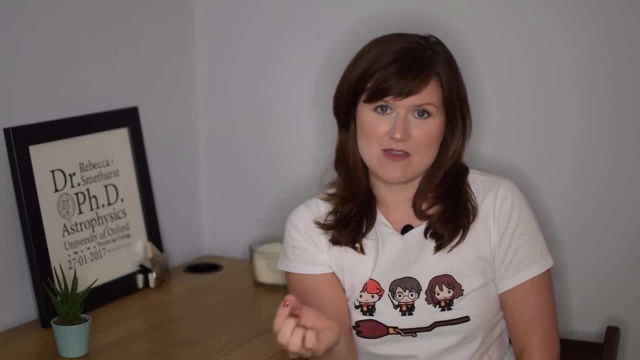 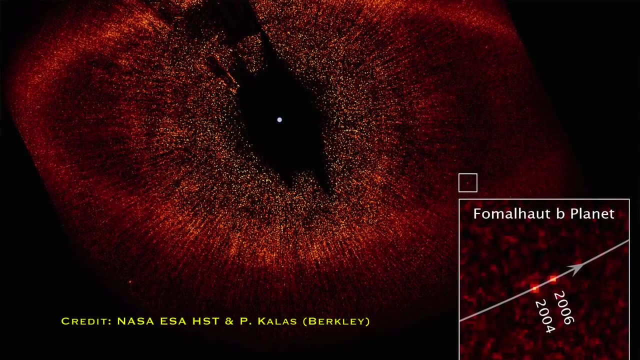 and noticed: oh, that little bright spot there, maybe that's a planet. Took another image in 2006 and saw that that bright spot was a planet. And they took another image in 2006 and saw that that spot had moved on its orbit around the star Formholt. This image is one of the most famous. 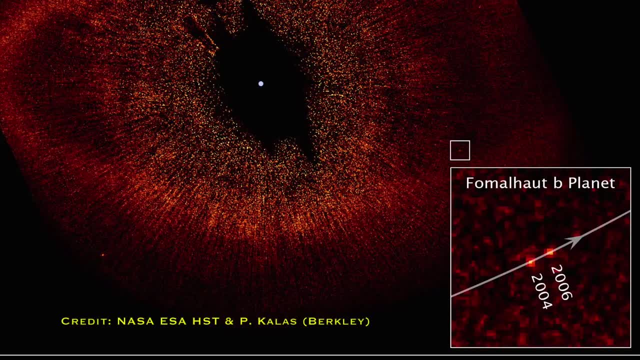 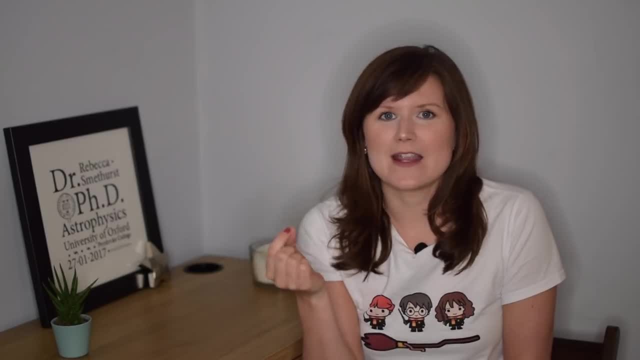 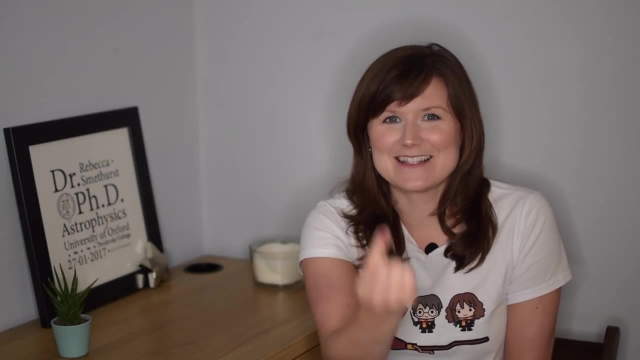 scientific images of the 21st century. It is momentous in its achievement. The fact that they've been able to detect something that is so faint it doesn't give out light of its own, It's only reflecting its star's light. next to this blindingly bright star is incredible, And the 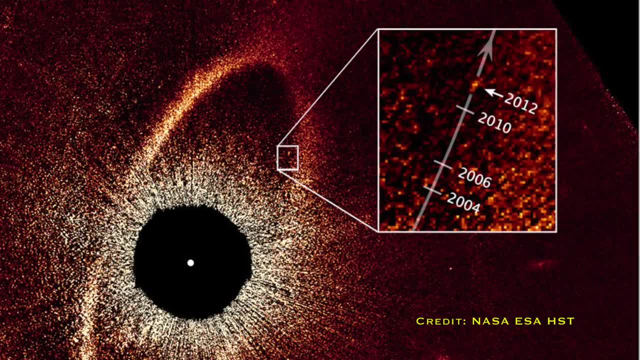 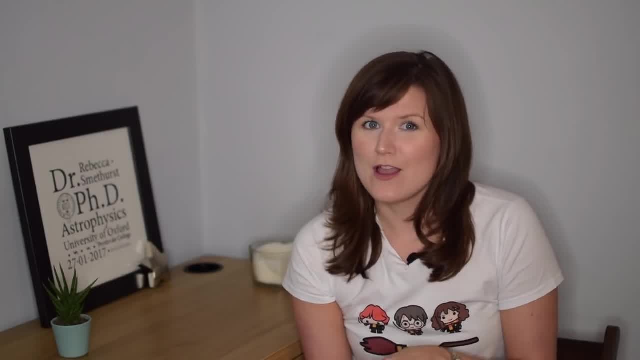 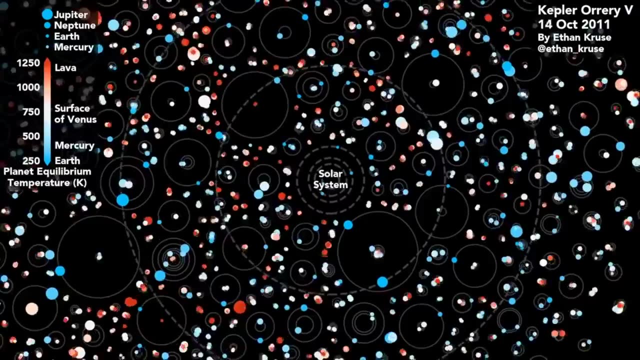 scientists were able to detect it, and they did the exact same thing and found it's moved even further around its orbit since we last observed it In the end of the decade, in 2009,. so the launch of the Kepler space telescope, a mission that would go on to detect 2662 exoplanets in its 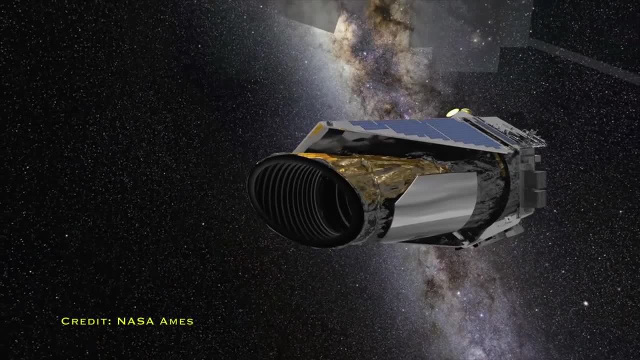 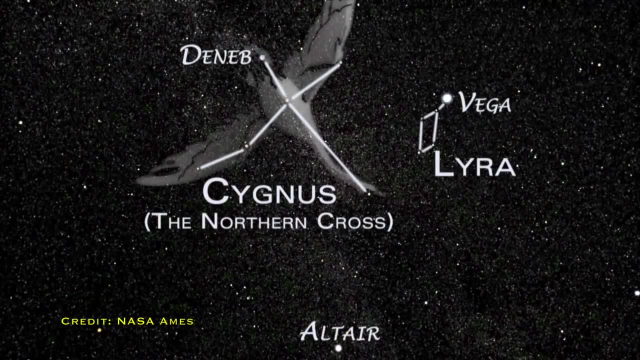 nine and a half years of service To detect those planets. the Kepler Space Telescope stared at the same patch of sky for that entire time in the constellation of Cygnus, And it was basically recording constantly the brightness of those stars, looking for those dips where 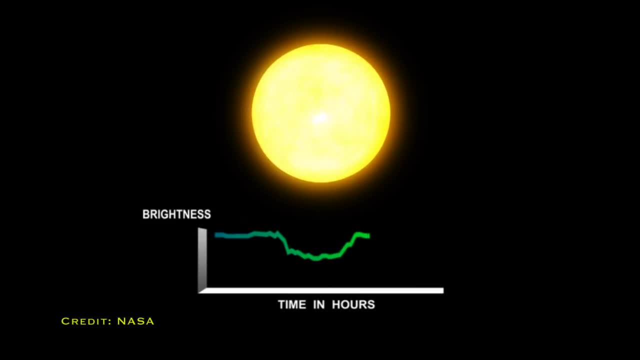 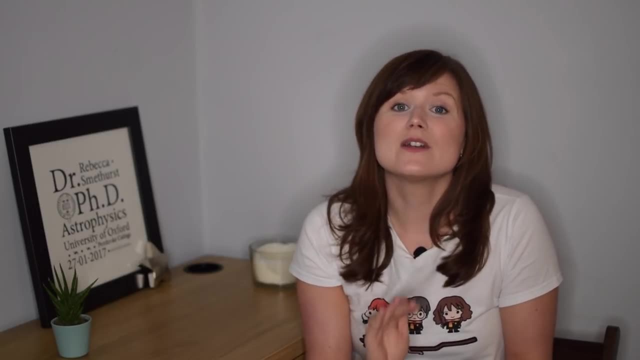 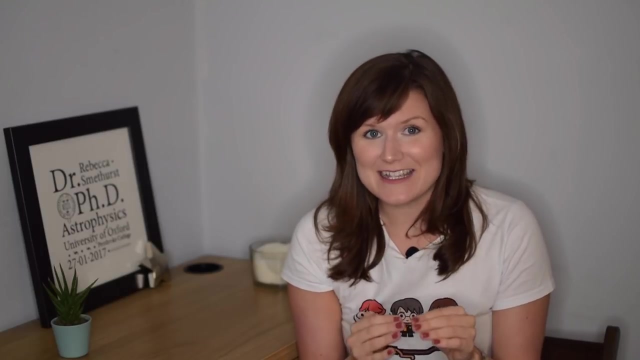 there would be a transit of the planet in front of its star. It was a phenomenal group effort by NASA and ESA that allowed that mission to happen, and its legacy will continue to live on in the decades to come. 2014 then saw the detection of an Earth-sized planet in a habitable zone by Eliza Quintana and 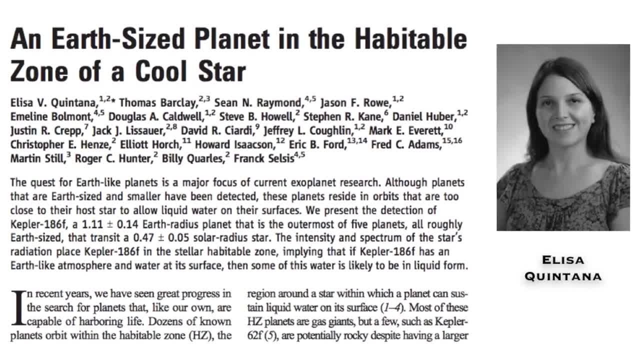 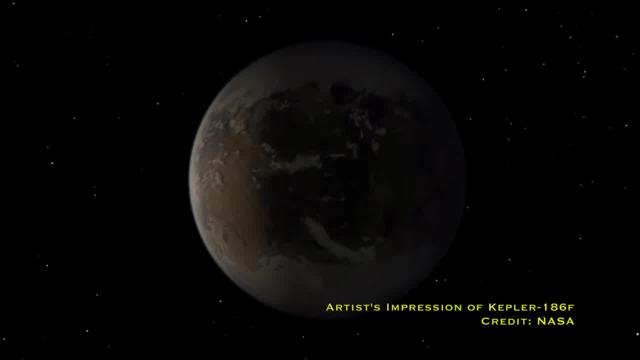 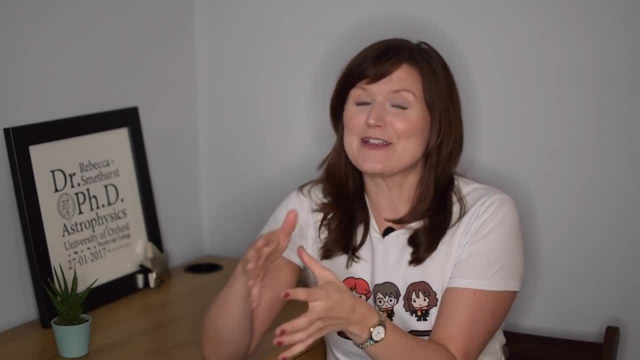 collaborators. Kepler-186f is 10% bigger than Earth and is the outermost of a five planet system, all of which in the habitable zone around their star, And that was the most Earth-like planet that we knew up until 2015, when the mantle was stolen. 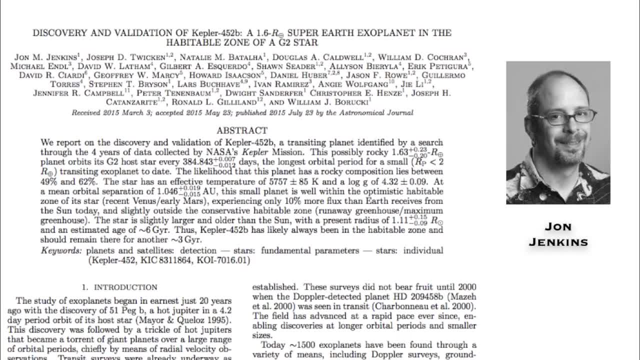 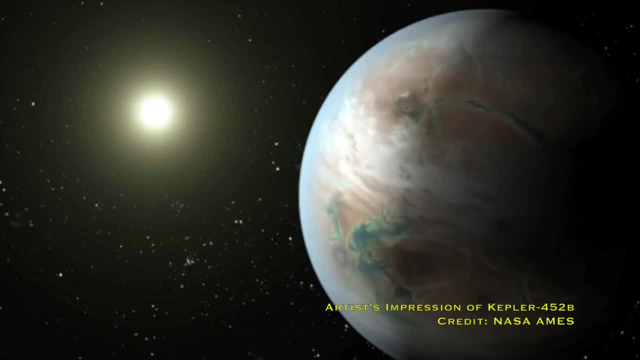 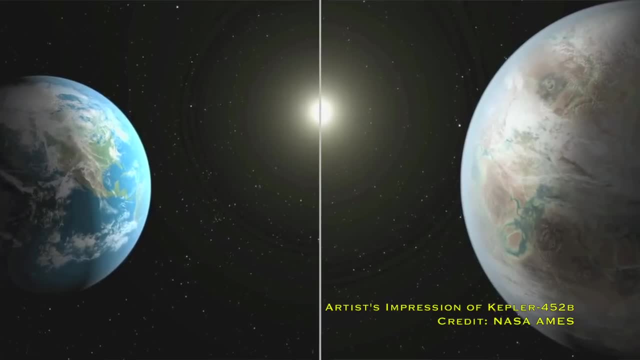 When John Jenkins and collaborators discovered Kepler-452b. This is a planet that's just over 50% bigger than the earth Earth, but it's orbiting a star exactly like the sun every 384 days, And that puts it well within. 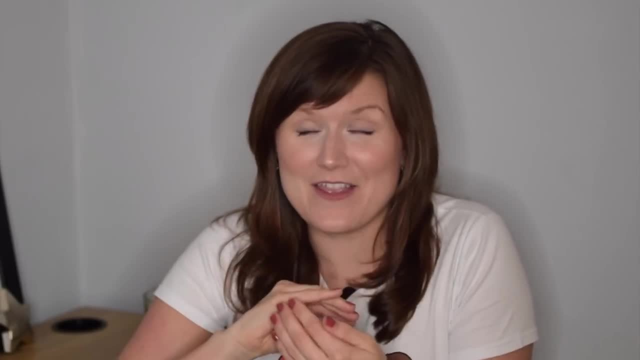 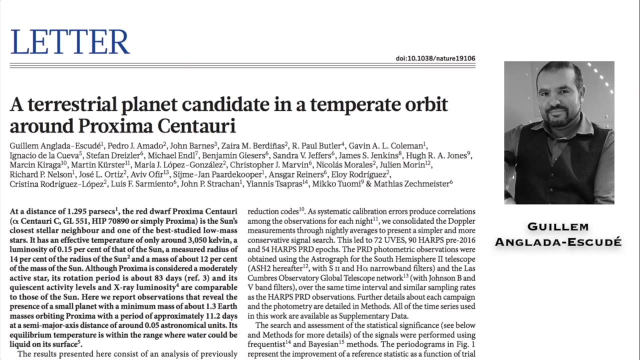 its star's habitable zone, And so all of those properties- the fact that it is so similar to Earth- have earned it the title of Earth 2.0.. Then, in 2016,, Anglada Escudé and collaborators discovered the closest exoplanet to Earth in Proxima b. This was a planet orbiting Proxima. Centauri, aka one of the closest stars to Earth in the Alpha Centauri triple star system. Not only that this planet is about 30% bigger than the Earth, but it orbits a lot closer to its star, so much that its orbit only takes it 11 Earth days. So you would think that it would be. 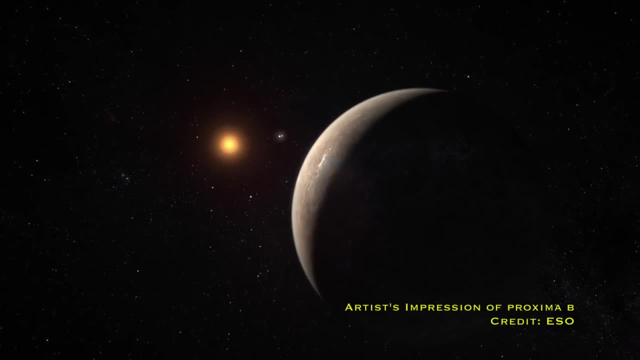 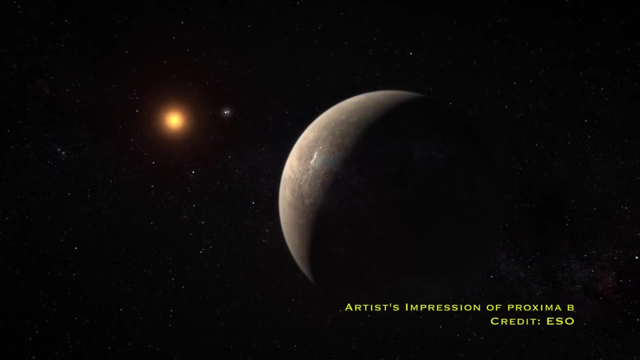 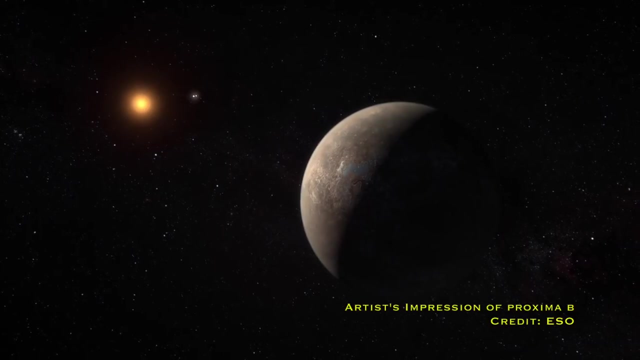 scorching hot. However, its star is only a red dwarf star. It's a very small, much cooler than the sun star, And so this planet is actually in the habitable zone as well. So not only do we have the closest exoplanet to Earth, but the closest exoplanet in the habitable zone as well. Then in 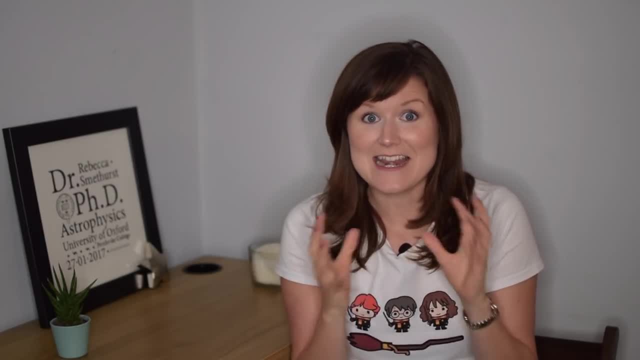 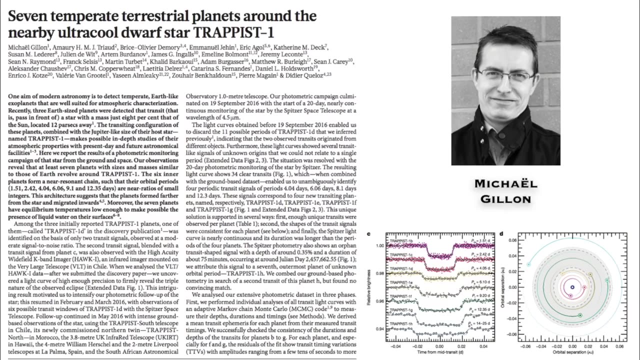 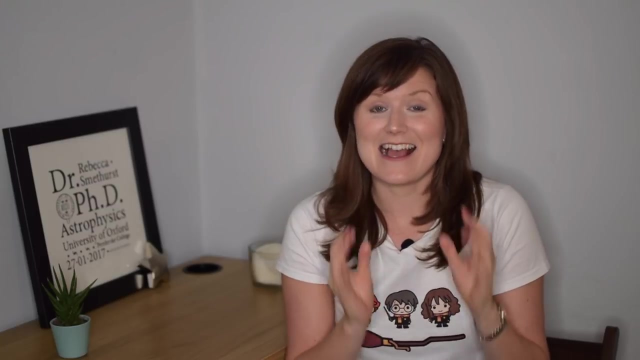 2017,, the record for the number of exoplanets in a single system was broken twice in quick succession. First of all, Gilon and his collaborators announced that they had found a seven-planet system around the star Trappist-1,, all of which were rocky planets, and in the habitable zone around this dwarf star again. 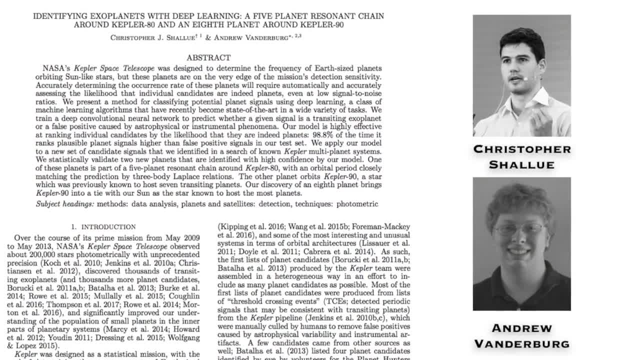 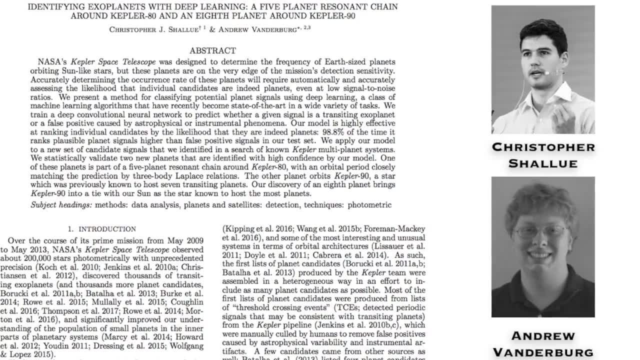 Then, later in the year, Shalhoub and Van der Berghe announced the discovery of an eighth planet around Kepler-90,- Kepler-90i. This made it as big as the solar system and the biggest exoplanet system in the world. So this is a very, very big discovery. So this is a very, very big. 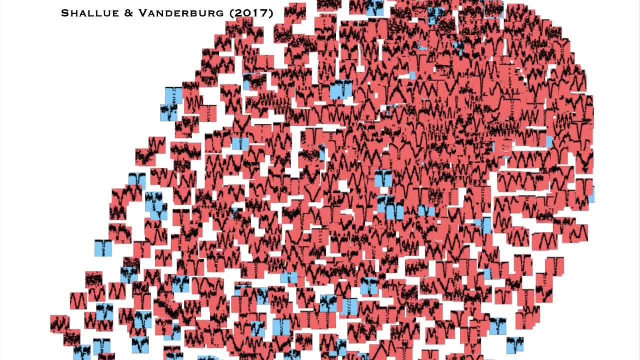 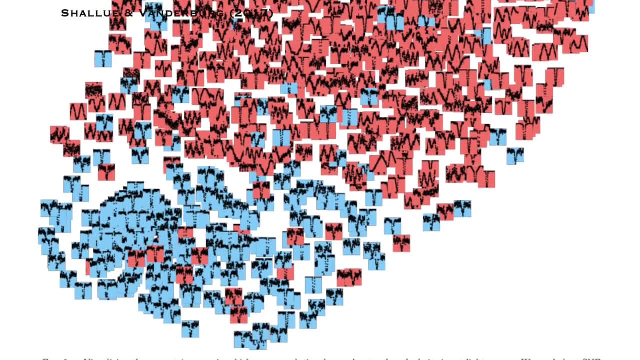 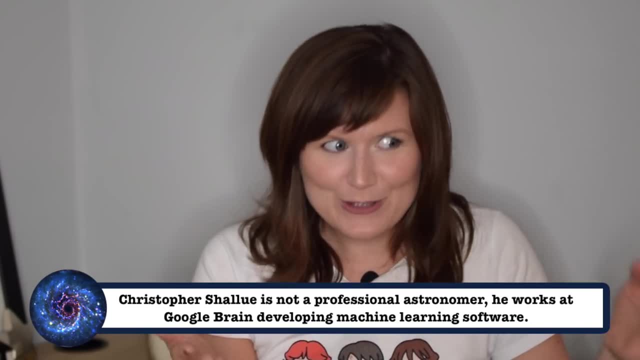 discovery And the country was very, very excited looking at it. This is one of the first eyelid testing efforts to discover food" And, departed from the chemistry of OKC, they tried to find one of the Earth's truth: separatists, also known as Kepa. 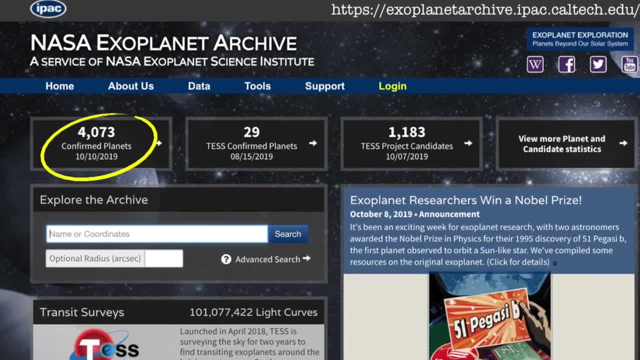 The cutthroat-smart 수 motherfucker Huawei. Earth scientific calls the first exoplanet that was discovered by machine learning, But it was also a landmark discovery, because the planet Kepler-90i was discovered in the data using machine learning. It was an algorithm that had been developed by the team at Google Brain, So not only like the biggest exoplanet system known, but also the first planet that was discovered by machining. Then, earlier this year, in June 2019, the number of known exoplanets went over 4,000. for the first planet, The TerraPlanet công hips suspärenja tells his talented quasirs, antioxidants for Nickels oppżenia not as seven. seeing the 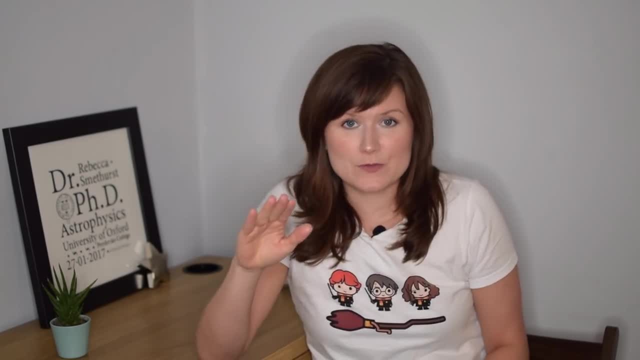 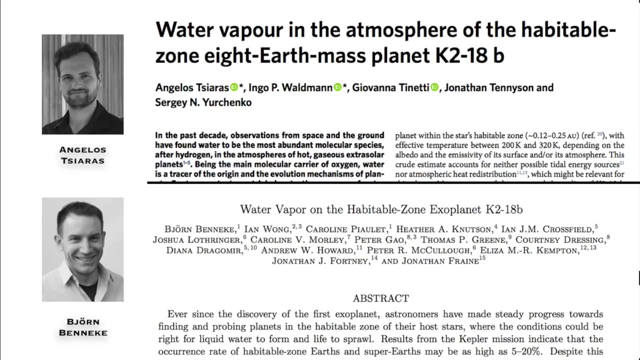 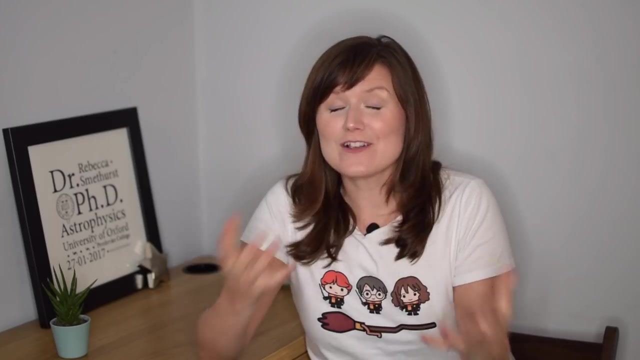 for the first time. Then, in September, two separate groups, one led by Tsaris and one by Beneke, announced the first detection of water vapor in an exoplanet's atmosphere that was in the habitable zone around its star. So because this planet was in the habitable zone, it was. much more likely that this water would be liquid rather than vapor form. This planet was K2-18b and it was very much a mini Neptune. It wasn't earth-like at all. it was a big gas giant. its atmosphere was mostly hydrogen, but it was still the first planet detected with water in. 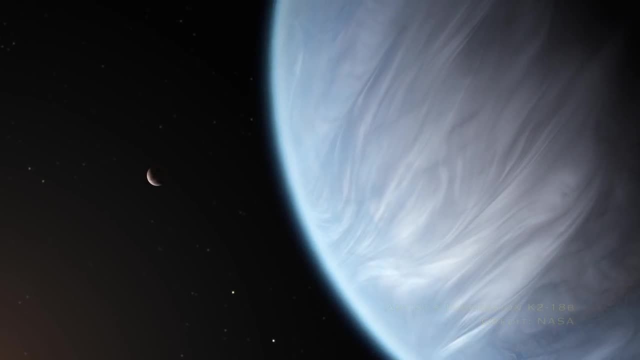 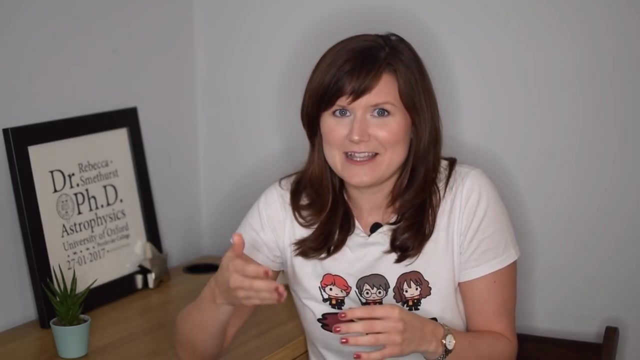 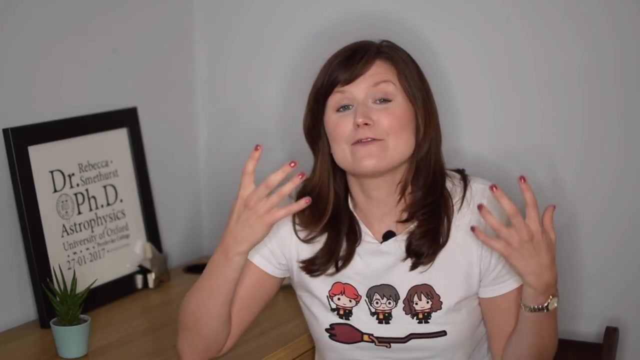 its atmosphere in a habitable zone as well. The obvious next step to me is detecting water in the atmosphere of an earth-like planet in a habitable zone. you know, water in the atmosphere of an earth 2.0, where you can imagine perhaps also it would have lived. 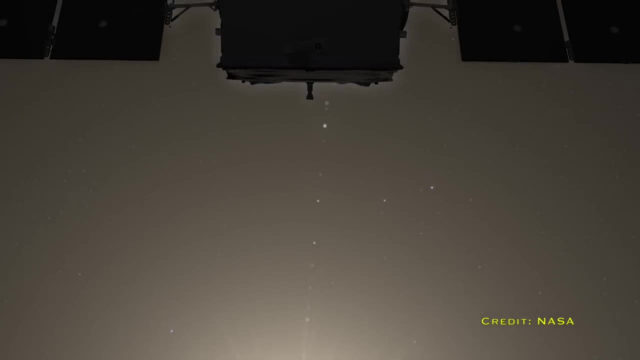 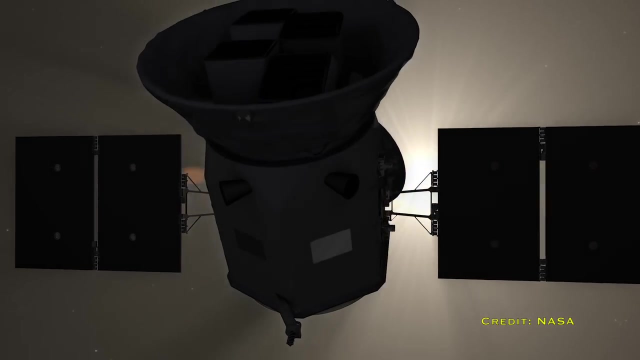 The next step I'm going to talk about is the discovery of liquid water oceans. That will probably come with the launch of the TESS mission in 2018, this is the follow-up to the Kepler Space Telescope, which has already facilitated the discovery of hundreds of exoplanets, and, with the 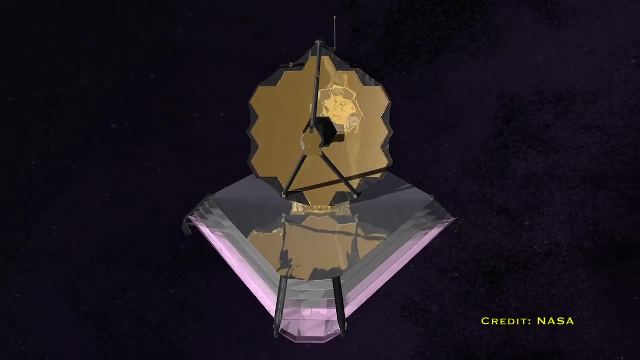 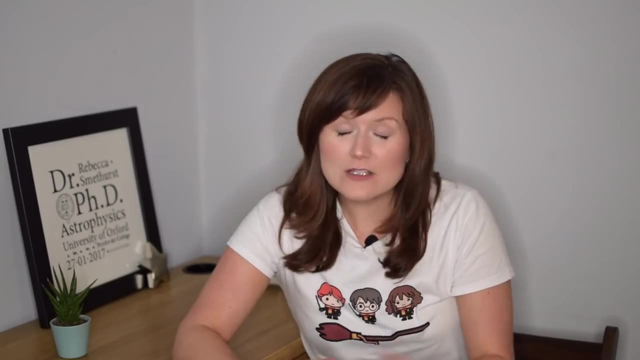 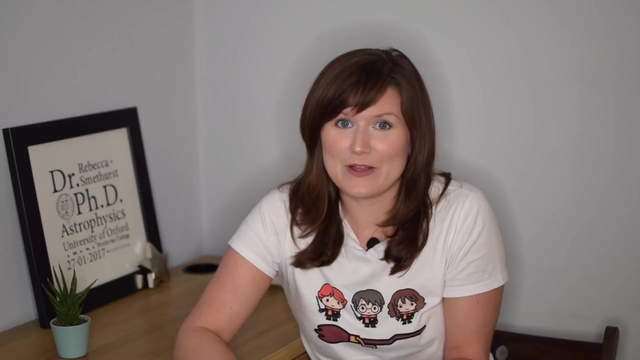 launch of the James Webb Space Telescope, which is the follow-up to the Hubble Space Telescope, which will allow us to get a much more accurate and precise spectra of these exoplanets in the infrared, where this water absorption takes place- tip of the iceberg in this field. that was fully made possible by that first. 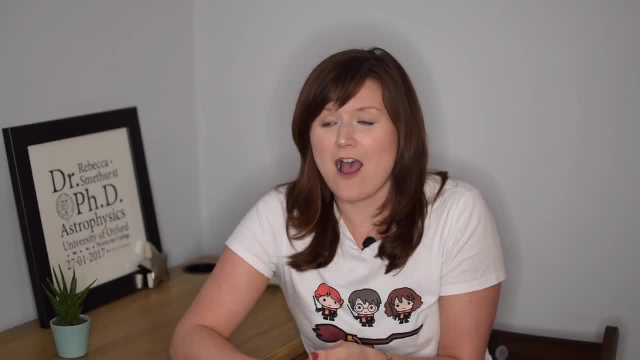 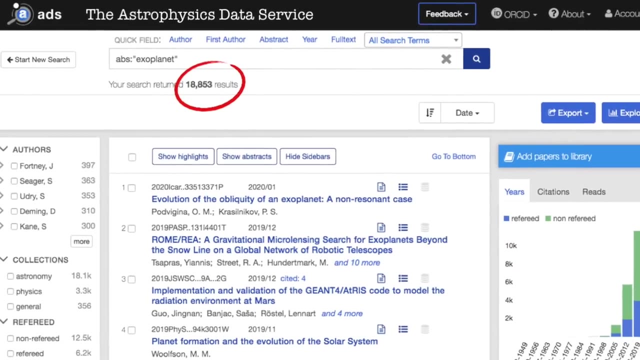 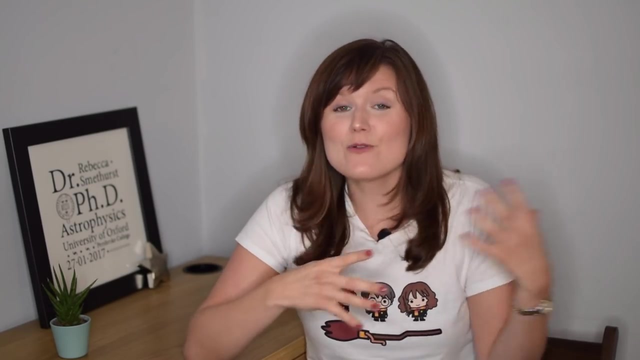 discovery in 1995 by Queloz and Mayor. I might have mentioned 50 or so results in this video, whereas in reality the number of scientific papers in this field must be in the tens of thousands. It's that legacy, combined with our new 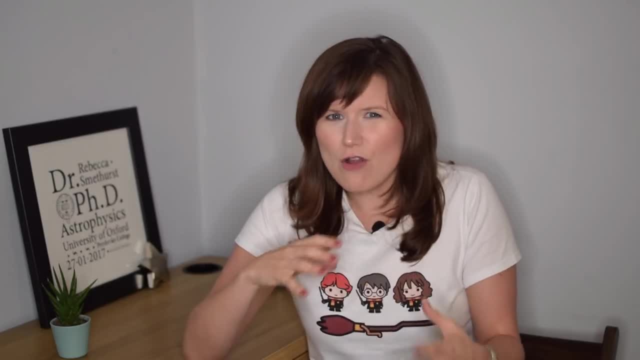 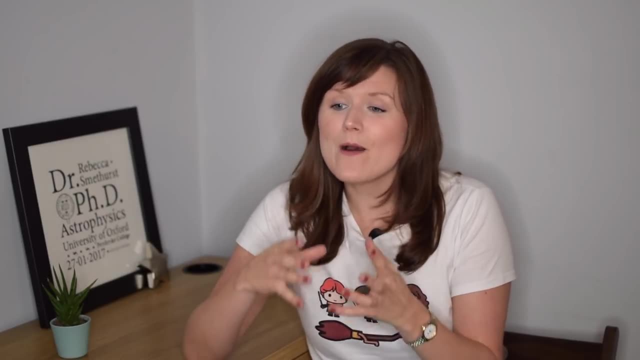 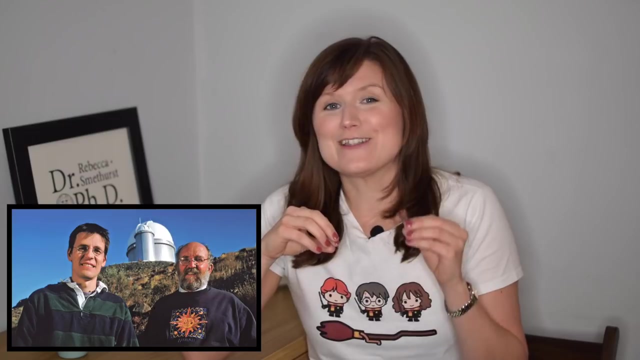 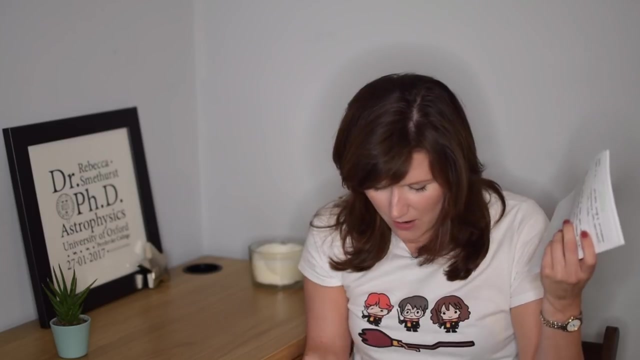 understanding of the fact that the solar system and Earth are not unique in our universe. that prompted the Nobel Prize Committee to award the Nobel Prize in Physics for 2019 to Queloz and Mayor, even 24 years after that first world and life-changing discovery. Oh, I didn't even mention Planet Hunters. What am I doing? 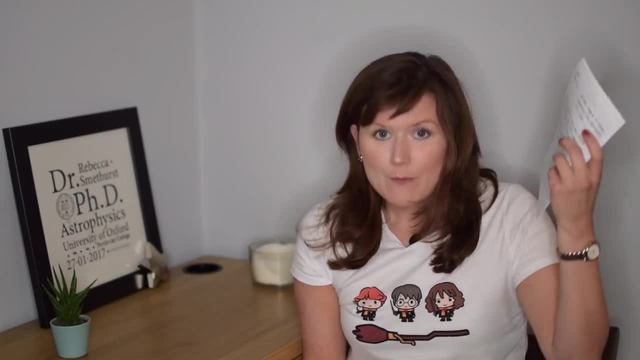 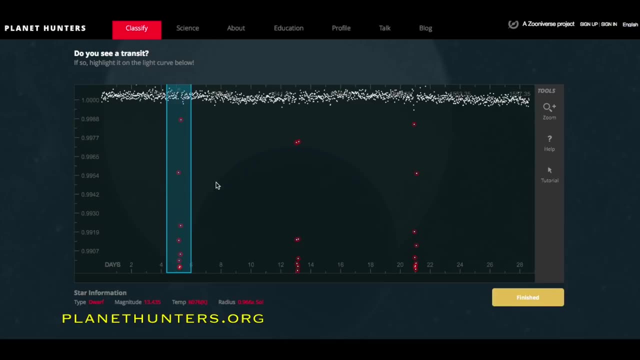 Oh my god, that's been running for years: Planet Hunters. it's a website that lets you search for exoplanets in the data, so all of the data from the new test mission will go online and you'll need to search through it to try and find the stuff that. 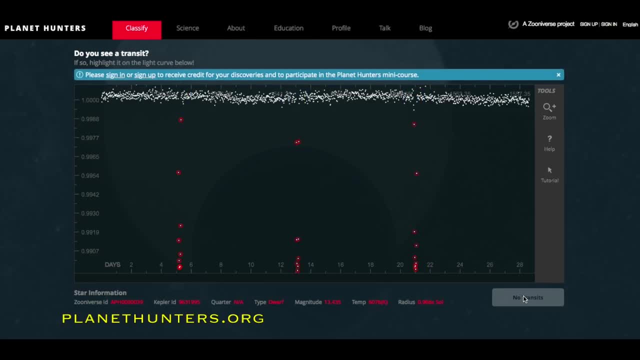 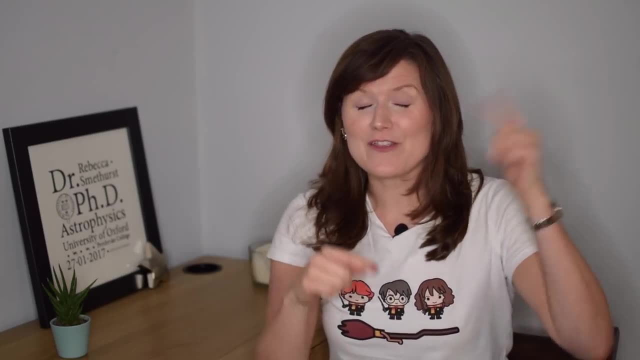 computers and algorithms miss, because you can only teach an algorithm to search for something that you know. What about the stuff that we don't know what it looks like? So I'll put a link in the description below if you want to take part in that, because it's a really cool project. 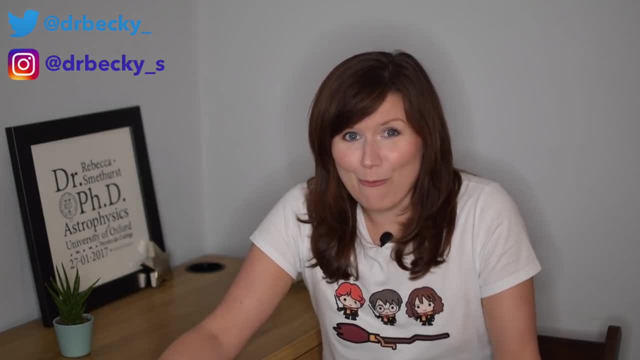 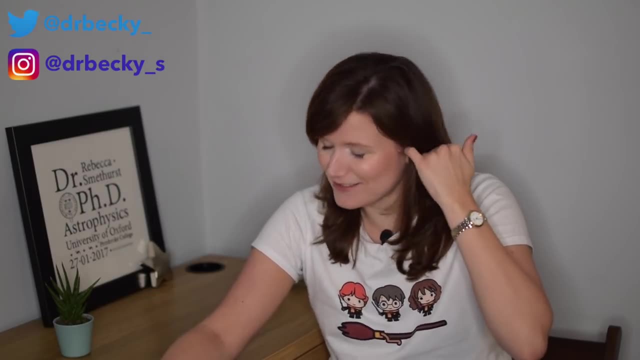 I wondered why on earth did they wait so long to award them the prize? I went fade, Don't spray it, Spray it, don't spray it. Oh god, this is going to be a good day already, And the publication of Isaac Newton's Principia in 1754.